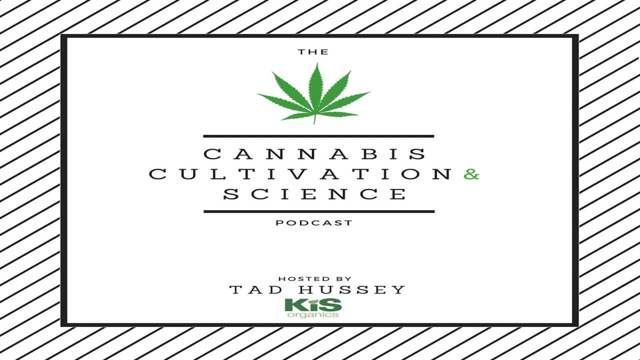 greenhouse gases. Her expertise is in helping people identify and remediate soil contamination in urban gardens. She has a passion to help others to understand the impact of heavy metals on the health of soils and the best way to improve soil quality. In addition to her appointment at 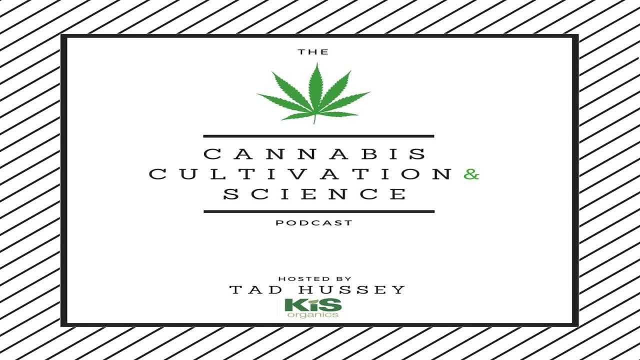 the University of Louisiana at Lafayette. she has taught at New York University, CUNY, Brooklyn College and the New York Botanical and Brooklyn Botanical Gardens. This has led to her creating the Delta Urban Soils Laboratory at ULL that provides soil. 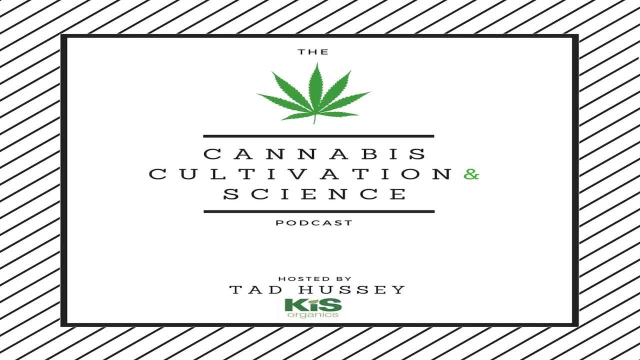 testing services and informal education to communities and businesses across the country. Now on to the show. You know listeners. a little bit of background into who you are and what you're doing, Of course. So I am Dr Anna Paltseva. I'm also known by Anya, which is a Russian nickname. 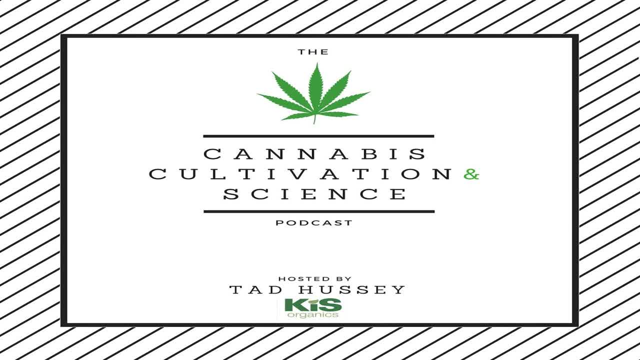 I grew up in Russia, in the south of Russia, in my parents' garden. I used to play with dirt when I was a child, And this childhood game became my career. eventually, My parents are agronomists and they taught me how to take care of soil, our land and grow. 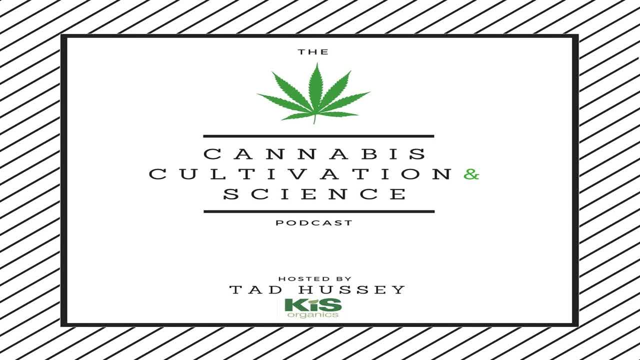 our own vegetables and food. So I brought my family trade to the next level by conducting research in urban soil, in urban agriculture, And I got my doctorate degree in earth and environmental sciences at the City University of New York Graduate Center A couple years ago And basically since then- well, for the last seven years since I started- 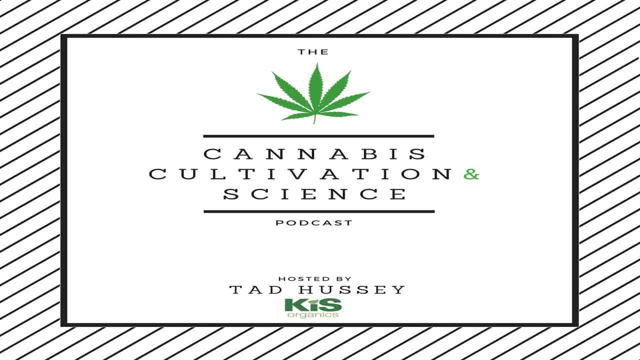 my PhD, I focused on urban agriculture, urban soil contamination and soil testing, which also led me to open up recently my very own Delta Urban Soils Laboratory at the University of Louisiana at Lafayette, where I'm currently an assistant professor in environmental sciences. 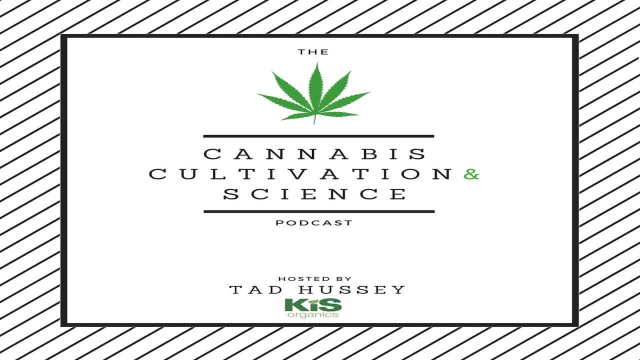 That's so wonderful And I think your area of research is just really fascinating. When we talk about urban soils, you know, trying to grow food in the city is really challenging And the big issue is soil contamination, related to you know things that we're dumping into the soils. 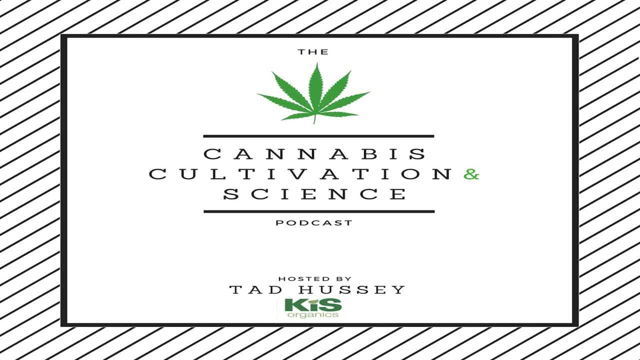 things that are leaching into the soils and these heavy metals. Can you talk about some of the other research that you did around heavy metals? Of course, yeah, So starting well when you- yeah, it started like 2013 when my PhD advisor. 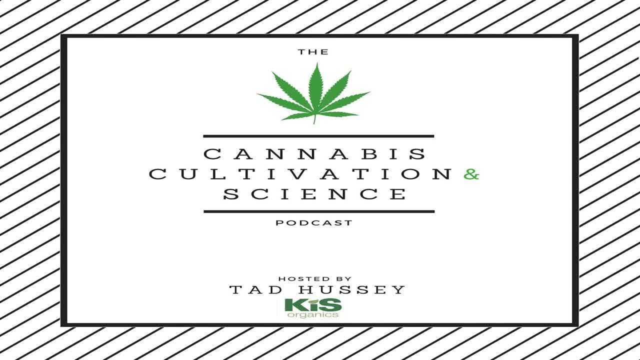 offered me to do a test on studying bioaccessibility of lead, And back then I didn't know what bioaccessibility was, But basically now I can easily define it as a fraction of harmful harmful contaminants or metals like lead that we determine in soil in order to understand how that particular 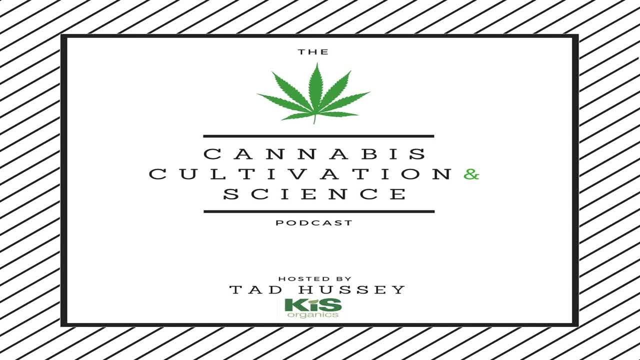 fraction can affect human health. So basically, what we find is that not all metals are harmful and not all total concentrations are harmful. So let's take lead, for example. If we find with a standard method that there is like 1,000 parts per million of lead in soil, It's a very 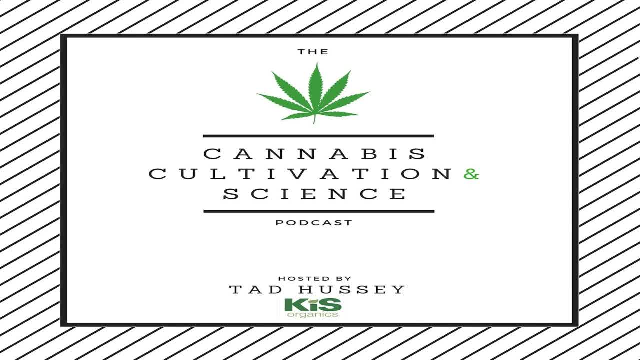 high number, but it doesn't mean that all of this 1,000 parts per million is going to be harmful for humans or plants. It really depends on what form this lead exists in soil, And this form will determine the bioaccessibility. It can be low or it can be high, Depending on chemical composition. it can be high or it can be low. So it can be high or it can be low. Depending on chemical composition, it can be high or it can be low. So it can be high or it can be low. So it can be high or it can be low. So it's really important to tell the chemical state of this metal. 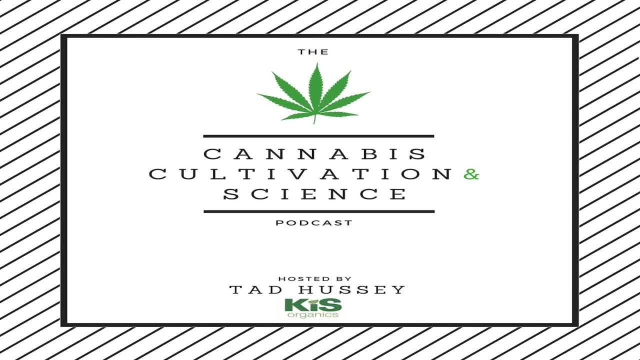 If it's lead combined with organic matter, with phosphate, it will be very stable. The bioaccessibility will be low. So lead will be present still in the soil but it's not going to be harmful- or at least much lower level harmful- to plants or human. But if it exists in the form of lead carbonate, it may. 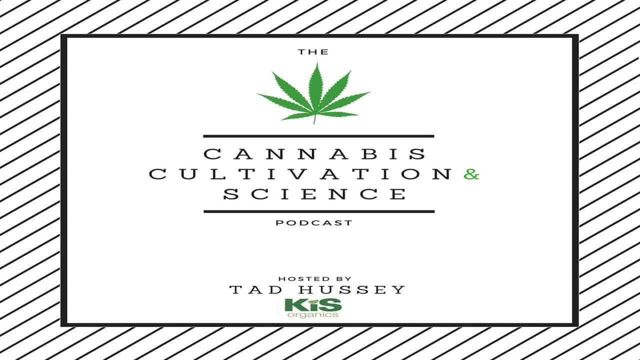 soluble in the environment, thus more harmful. so my research started with assessing different methods on, specifically on by accessibility of lead, and it led me to develop two different methods in collaboration with the columbia university research group and the university of molise in italy research group on how we use instruments to determine by accessibility of lead in soil. 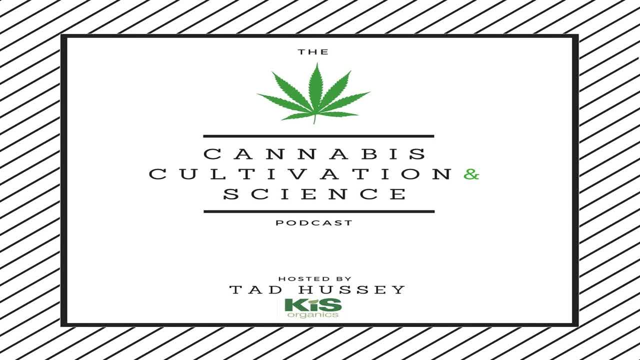 using x-ray fluorescent analyzer machine, and another one was visible near infrared spectroscopy. this method allow us to quicker assess the harmful fraction of the soil, not just total concentrations, and be able to test more soils, so samples, at a shorter period of time. so so what you're saying is: it's really. 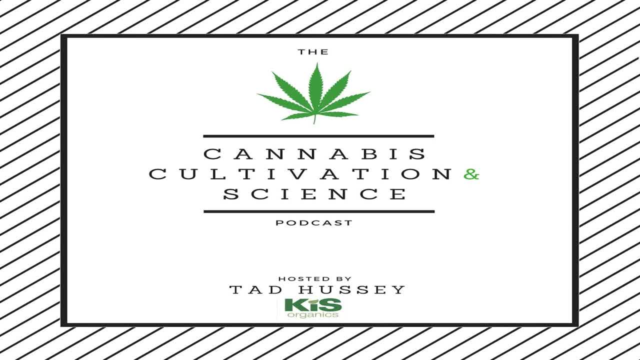 important to look at how bio accessibility in, in that how easily can the plant uptake that particular heavy metal? and um, one of the factors that you mentioned is the the form that that heavy metal is in the actual chemical form of that of that heavy metal, in terms of what it's. 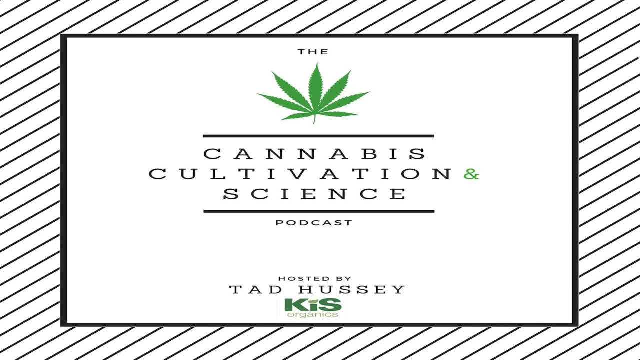 bonded to um. what are some of the other factors? like i just off the top of my head here, i'm thinking that plant selection would play a big role: ph, the, the hydrology, or the amount of moisture in the soil. how do all of these sort of come together in terms of determining um? you know, if you can? 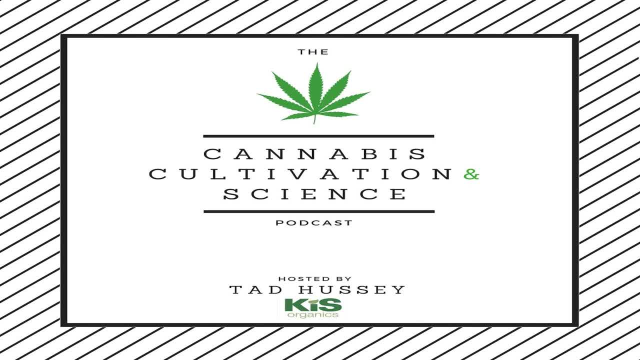 grow a safe crop in the in a given soil? that's a great question and all of those factors it did have a huge role in the availability of metals and soils and uh we found that a plant type is is actually more important uh than the amendment type that we tried to use to remediate soils. 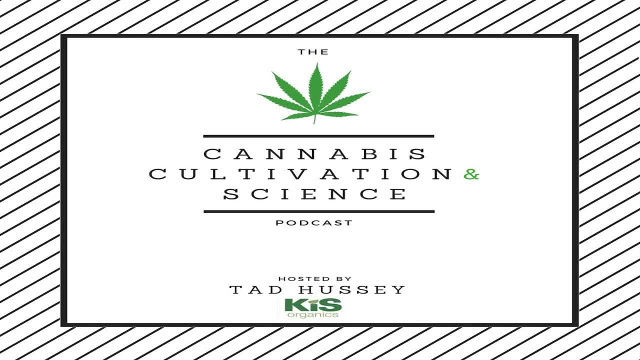 because plants would react differently. some plants would take up more lead and arsenic that we studied, some of them would not, or it would be more susceptible to the uh if those like we grow tomatoes or eggplant or squash. sometimes we can use really fresh tomatoes in microcontamination of soil. let's just cut some vegetables, uh for sort of in 400 yuan or 200 cents. 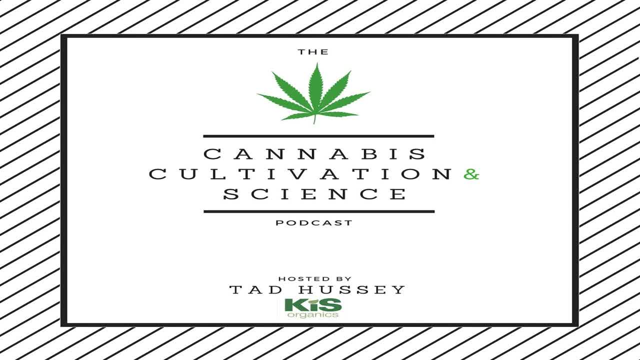 per feature from some of these kinds of tropical marketplace, so you can get either fish, still해 that it will be growing further from the surface of the soil because plants have physiological barriers inside of them, like fruit vegetables, And if they grow further from the soil then it will not have splashes from surrounding. 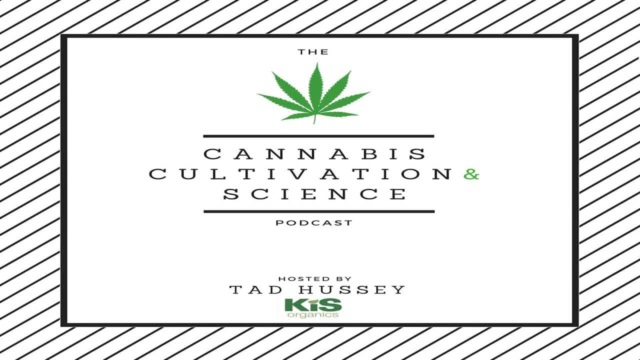 areas, And then leafy greens and then root vegetables will be, of course, more susceptible to this level of contamination. Another factor, like pH that you mentioned, which is really huge, is that most of metals will be least available at pH close to neutral. 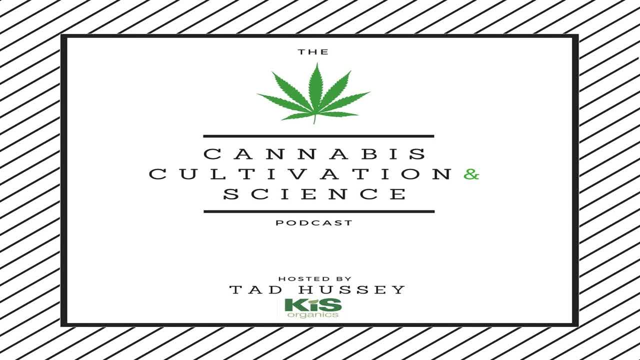 So, like slightly acidic to neutral pH, metals will be least available, while nutrients will be mostly available. So nature is smart, as I like to say. It makes nutrients available and metals not, Okay. But once it drops pH, drops to very acidic levels, it can make lead and arsenic for. 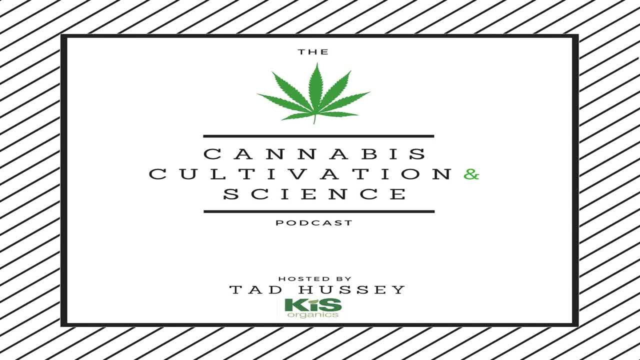 example, more available for plant uptake or human impact. So it's really important to keep pH close to neutral as possible. Organic matter is another one that's really important to mention because it binds lead or some other metals and forms organic mineral complexes, Which more or less is stable, and it will take time for organic matter to degrade to. 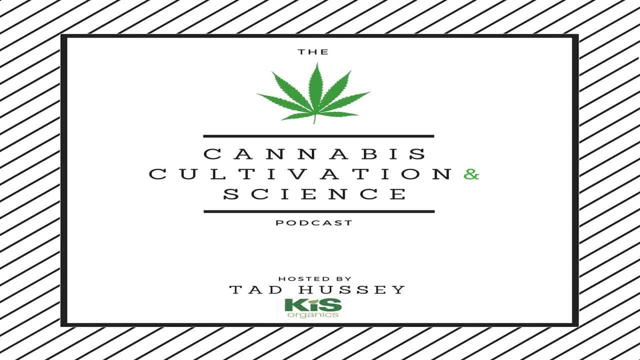 release those metals again. So we found it to be an effective way to remediate soils by adding compost to contaminated sites, And on top of that it also has a dilution effect. When we add the extra volume of compost or any other organic amendment to the soil, it 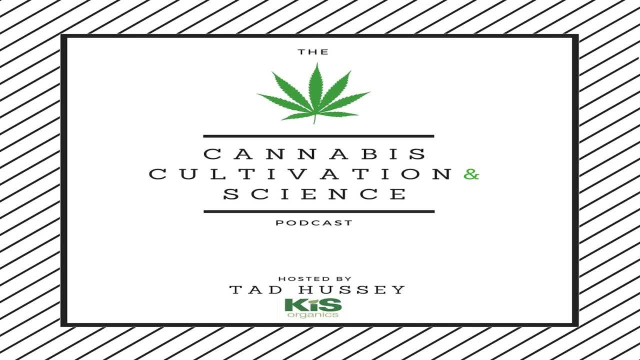 dilutes the overall concentration, And so we see that in most of these soil we have the same amount of water, which is the same amount of nitrogen in the soil, which is the same amount of nitrogen in the soil. So it also creates a second dilution effect in, let's say, tomatoes or fruit, or an eggplant. 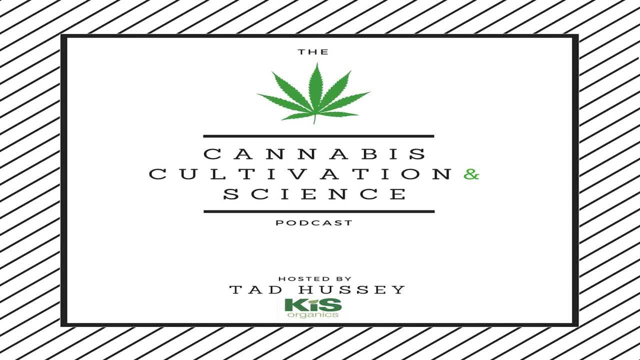 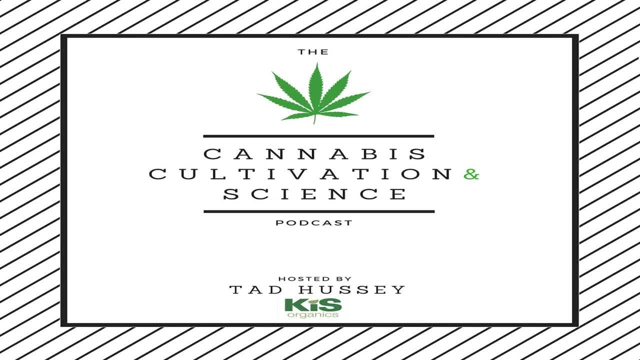 Indeed, it's good to have moisture in soil, especially if it's summer and it's very windy or it's an area that's susceptible to erosion. So moisture helps to reduce dust and redistribute contamination, So it's really good to have it. 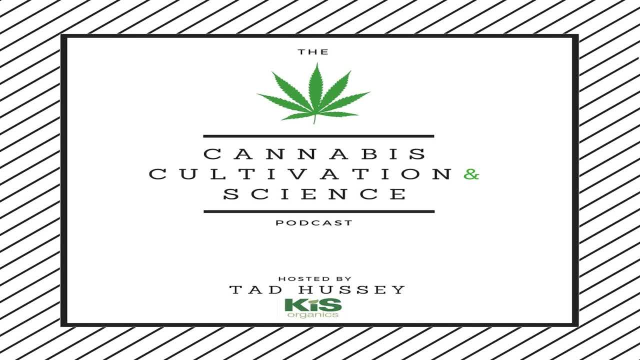 Another factor is soil composition. Is it sandy soil or clay soil? Because clay soils may hold more contaminants as much as they hold nutrients, while sandy soil is more permeable and that consists of pores, and pores doesn't really hold down much of nutrients or contaminants on their surfaces. 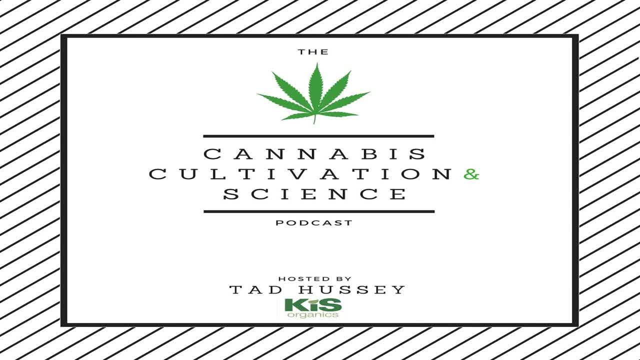 So there will be more leaching happening in sandy soils compared to clay soils. that will act like a sponge. So you're referencing the CE, The CE or cation exchange capacity of a soil, and the higher the CEC, the higher the ability to retain heavy metals in that soil. 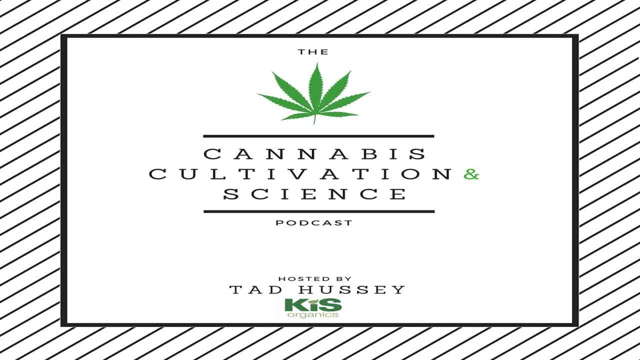 Yes, the cations, the positive metals, yeah, Yeah. and then what about the anions? though? In a higher CEC soil would you still see more anion retention? There's a possibility there will be leach out more. 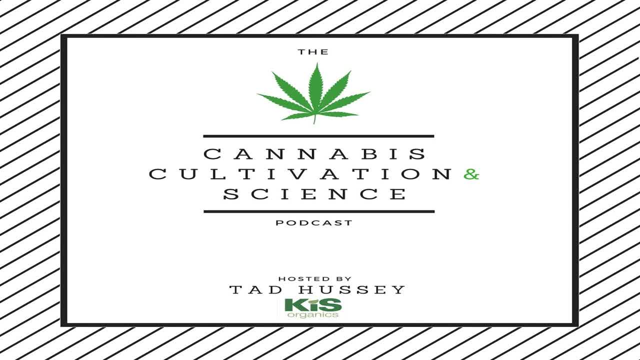 Okay, Arsenic is more leachable. For example, lead will stay in the soil. It's not very mobile. but arsenic, typically in a negative form, is arsenic or arsenite will be susceptible to leaching and moving down in the soil profile. 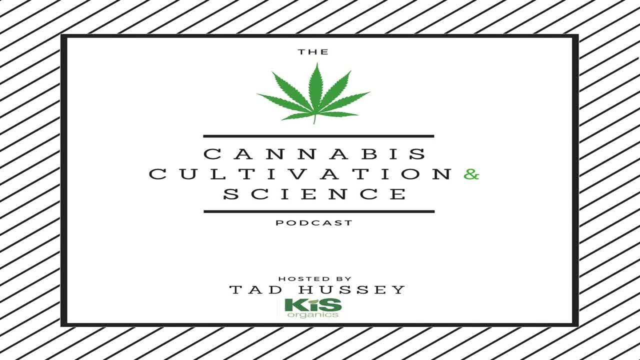 So you mentioned compost. Now I think of compost as a source of soil contamination, in terms of heavy metals as well, depending on where that compost is sourced, because I mean, frankly, locally, a lot of the municipal composts aren't really doing good testing. 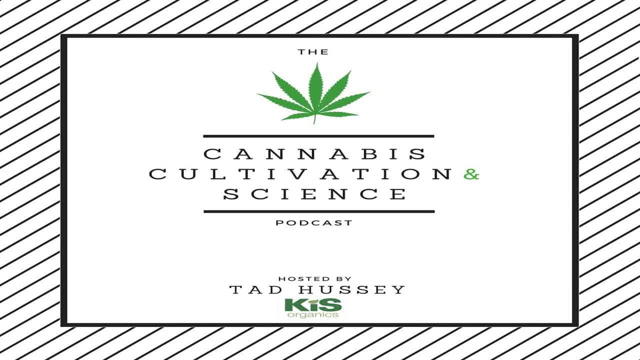 and they're composting some, you know, I think, somewhat mixed material, where people are throwing stuff into their yard waste that they shouldn't be essentially. So how does one evaluate compost to know if what they're adding is actually going to be decreasing? 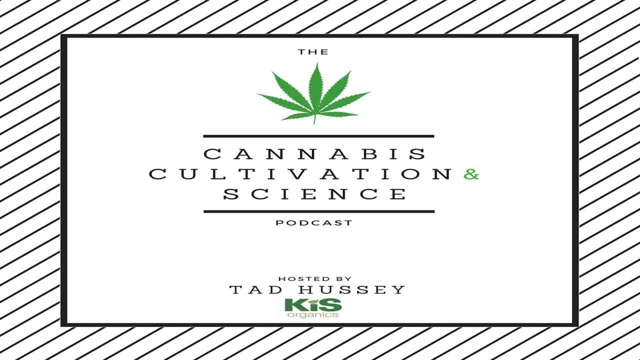 their heavy metal load or potentially increasing it- Great point. And we also found that some compost that we were buying for our research contain elevated concentrations of metals that shouldn't be there And, of course, we didn't use them for our research. 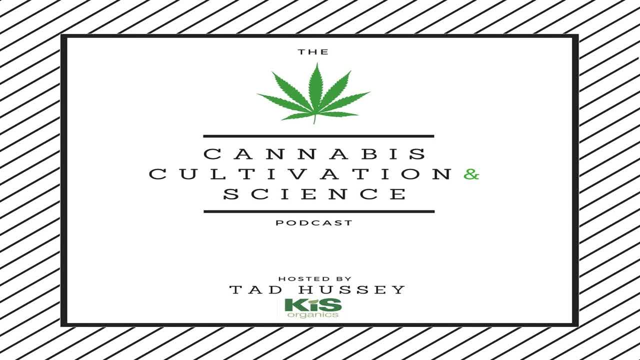 but it was a really interesting discovery To answer your question. basically, testing is important. You should periodically test the samples or bags of compost or any other amendment that you buy in the market, And it's a really good investment if you want to make sure. 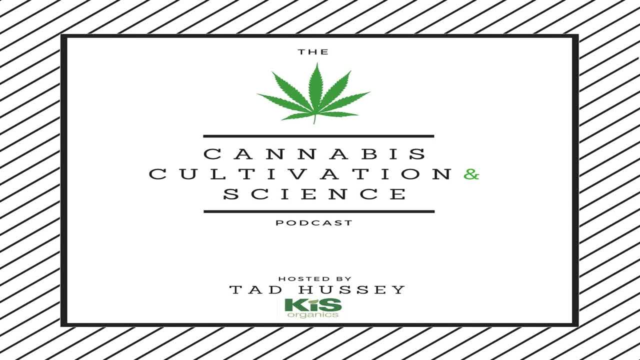 you're not adding additional heavy metal concentrations, You will still get some of the metals, because metals, you know they're present in plain tissues, but they should be at a low concentration, Unless those composts are made from contaminated manure or from trees. 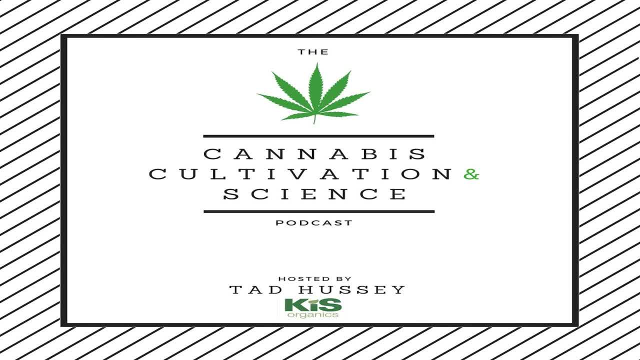 leaves from the trees that grow next to road, other type of compost. if it's like you make your homemade compost, it's going to have very minimal metal concentrations that shouldn't be harmful. So testing is really important to understand what levels you add into the soil. 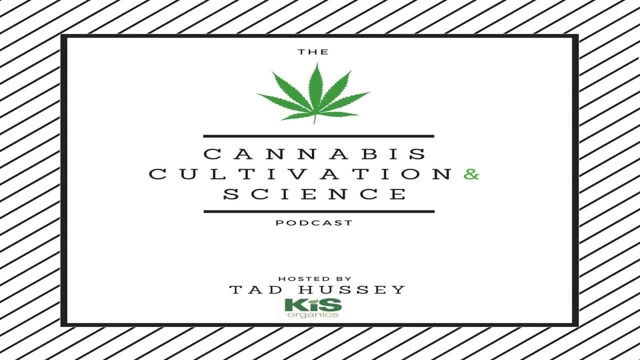 so you don't create accumulation of these metals, And I think that that's the answer. You either make your compost yourself and you know what you put in the compost, or you test what you buy And you know. so, for one of the things I want to talk about with you is: 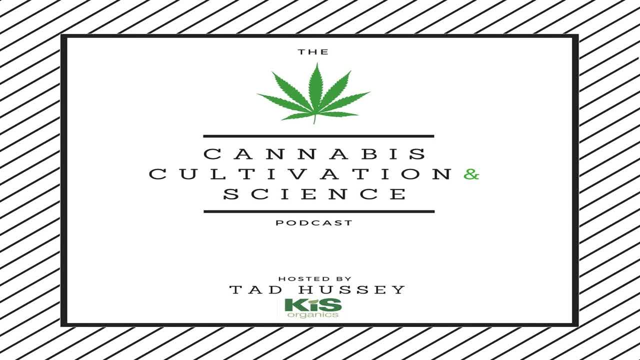 the fact that I agree testing is so important, but it's been it's been not affordable for people. It's been way too cost prohibitive. I know when I first got my soil mix tested a potting soil to make sure that we were meeting the requirements of a fertilizer. 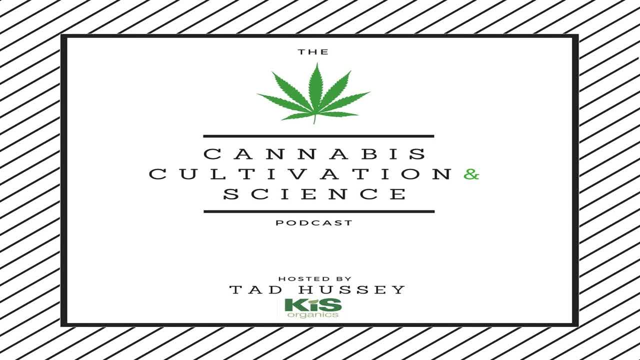 because of the amount of nutrients we're putting on, it's a much higher requirement. So if I were just going to sell potting soil, I wouldn't have to test it for heavy metals, And that's what 99.9% of the 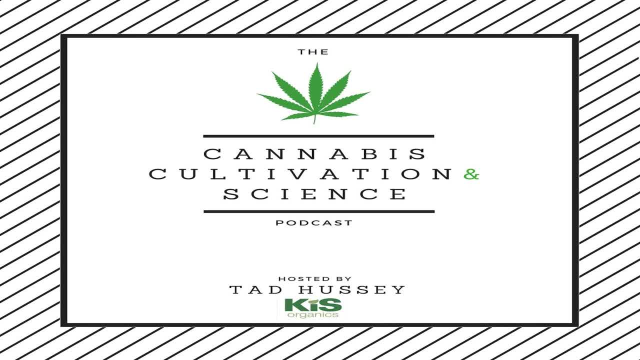 industry does right now, And so we don't really know what heavy metals are in our potting soils, because no one's testing them and no one's testing the vegetables. If you register as a fertilizer, it's a higher requirement. Anyway, long story short, the cost to do that was a few hundred dollars. 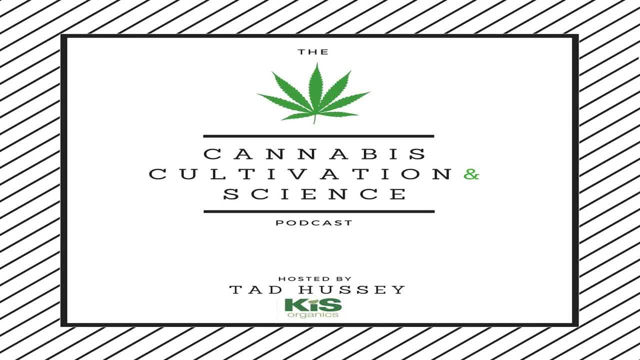 It was quite expensive And then I get a guaranteed analysis and then I can put this gets publicly published. But I agree with you, this is really important. But as a homeowner, I also wanted to test my soil in my backyard because I wanted to grow vegetables. 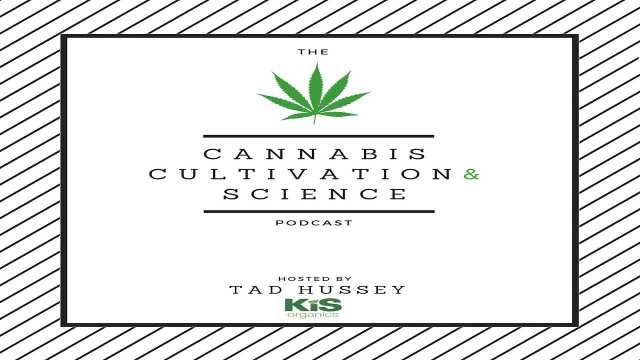 But being that it was a suburban area, I didn't know what construction had been done on the property before I bought it And I didn't know if things had been dumped here by a previous homeowner or things had leached. So talk to me about this lab testing that you're doing and the pricing and just how amazing this is. 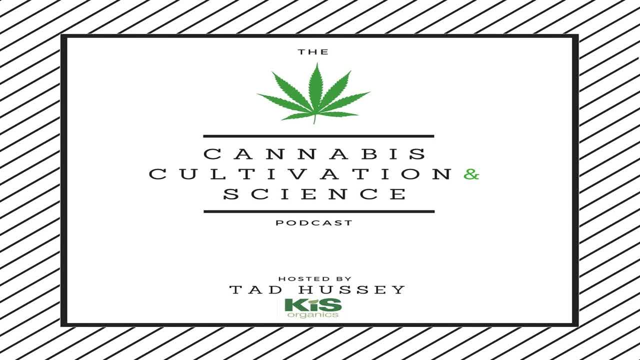 now as a way for people to test their soils. Yes, you brought up really great points. That's it. It's important to know land use history, land management history of your property And if it's possible to find those documents or maybe look up on some EPA websites. 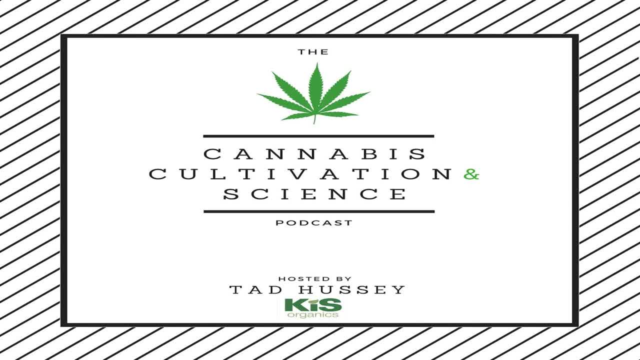 they always have really great toxic maps or information on the area So you can get an idea what potentially could be in your soil and see the proximity to highways or a former industrial site. At least get an idea what could be found in your soil. 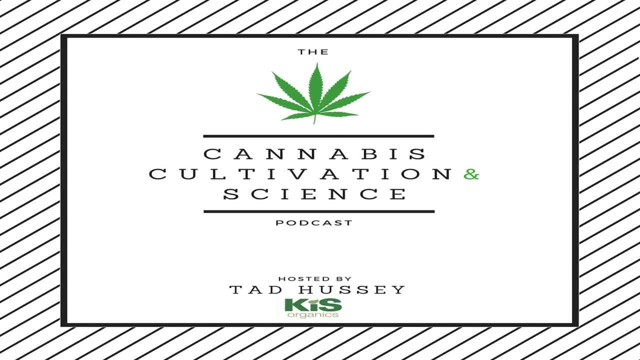 In terms of testing in the labs, of course commercial laboratories. they would charge certain amounts of dollars for their testing. Typically, university labs are much more affordable. From my experiences working in New York and Brooklyn College and here in Lafayette, we are not doing it for profit. 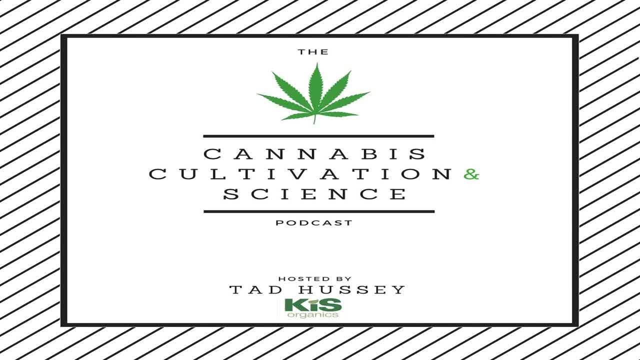 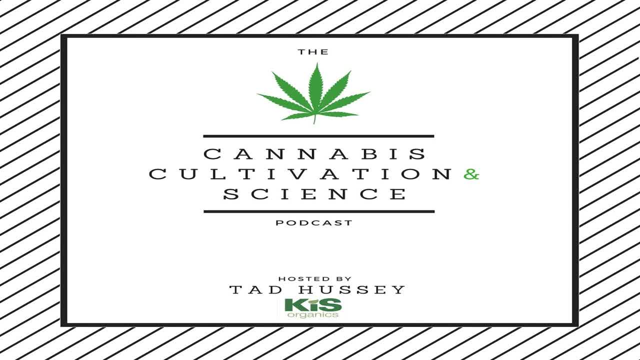 We use this for our own purposes- Expenses or costs to cover the materials we use to test the soil, And we support students. So the methods we're using, for example, to test heavy metals, is an express technique. It's actually called portable X-ray fluorescent analyzer instrument that we use a lot in New York. 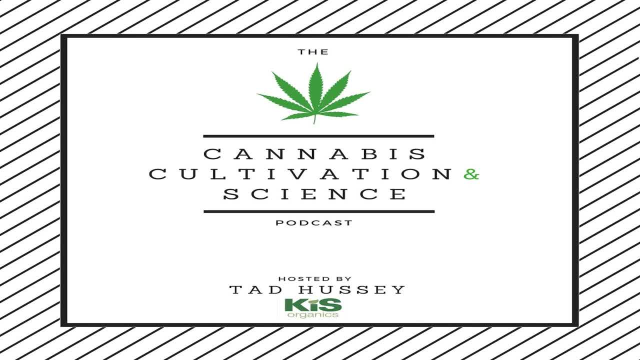 It's actually called portable X-ray fluorescent analyzer instrument that we use a lot in New York And we have here in Lafayette, And it reduces the cost because the machine itself is much less expensive than mass spectrometers that commercial labs typically use, And those mass spectrometers of course provide high accuracy and precision. 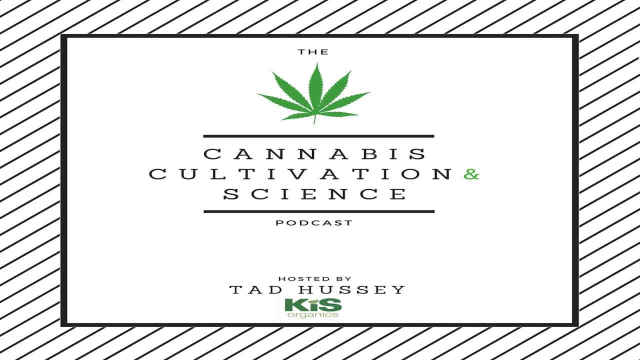 But modern XRF machines. they have actually good results, They're very reliable. They're very reliable And for samples they're properly prepared. And the way we achieve this relative accuracy is by, let's say, using the soil sample rule. 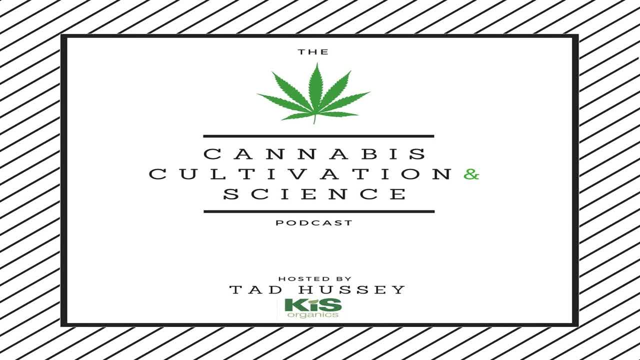 we'll analyze it by first drying in the oven, reducing the moisture condition. get rid of the moisture, Then sieve it to a millimeter size to create the homogeneity of the sample, And then measure this soil in special cups with a special film that does not have impurities on it, on this XRF machine and 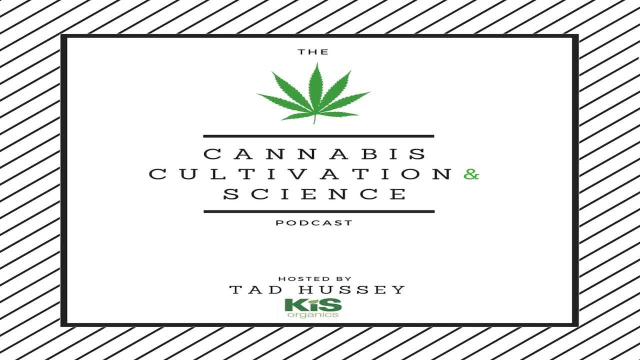 it's a result that give us close proximities to the mass spectrometers and this reduces the cost, because the instrument is much less expensive than mass spectrometers and it requires less time to prepare and analyze soils, because when you do a mass spectrometer analysis it takes a few days. 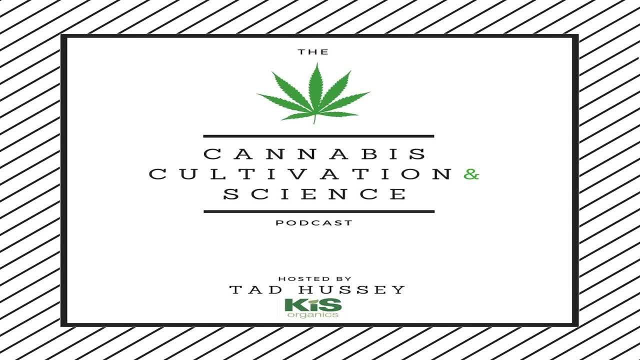 and you have to prepare the sample like dry it, sieve it through. then you have to weigh it very small numbers like 0.2 or 0.3 grams, and then you have to add different acids to it. so you have to put it in a microwave or in a hot plate and then you have to run it on mass spectrometers so it will take several hours. Then you have to process the data, so all of this will require more time and of course it becomes more expensive when you have to pay for the time of the lab. technician acids for machine SPMS. maintenance is quite expensive. 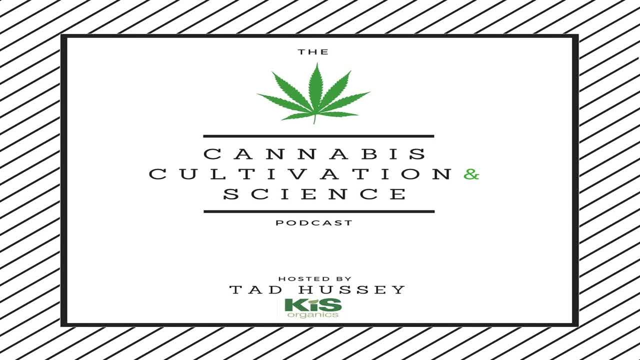 So what we have been using here is this XRF portable machine that allows much faster results and less time To process the soil samples. it can be also fertilizers, it can be different amendments- compost some sort of solids that we can analyze in those XRF cups that they call the smaller. 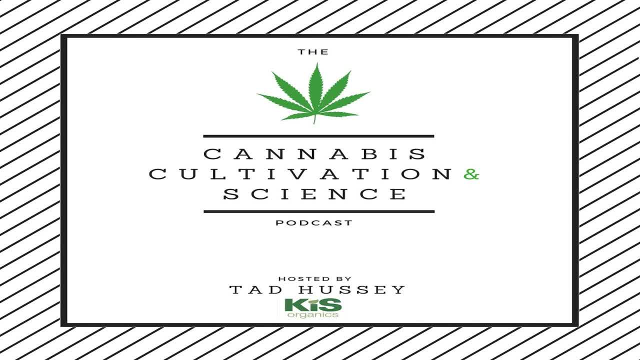 plastic cups that we use for the machine and we need typically at least like one centimeter depth of soil. Okay, And then we have to use the material to analyze it. So, if I understand you correctly, you're saying that the methodology that you use is maybe? 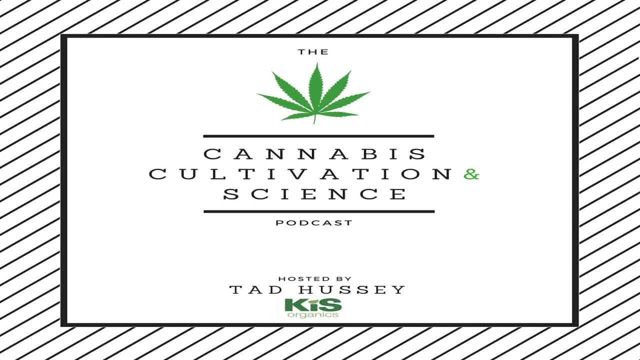 not quite as accurate as a mass spectrometer, but it correlates well. so it will give you, within a fairly good standard, deviation of what you would get from a mass spectrometer, but the method itself is dramatically less expensive and much faster. Exactly, Yes. 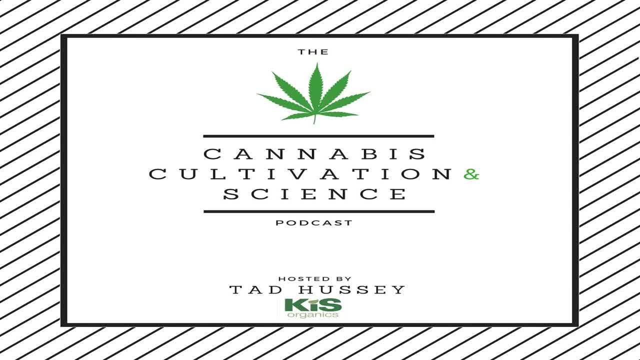 So it's just a huge savings in both time and money. So we've been using your labs now for a few months, testing, you know, formulations for fertilizers as well as our potting soils. I haven't tested any actual soils with you yet, but that's something I'm looking forward to in the future too. 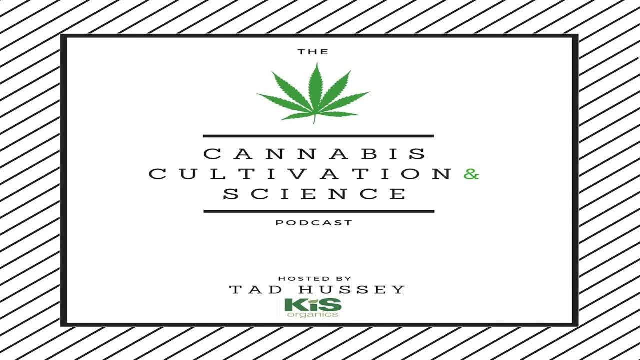 But you have the ability to test all of these things Correct, Yes, And also it's a good point too. Yes, It's a good point to notice that these procedures like having it slightly less precise and accurate than mass spectrometers, but you can test more samples with this for the same amount. 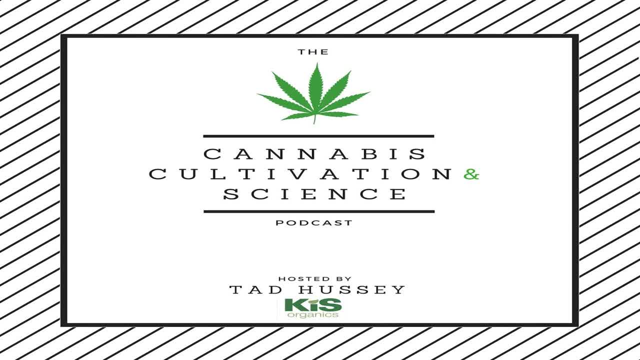 of money, you could test more samples and it will resemble variability of your soil or potting mix or whatever you're doing, because soil typically is very, or soil mix is very heterogeneous and soil in general is super heterogeneous At your property, your soil on the lawn versus soil next to the foundation of the house or under a tree or in your vegetable garden. 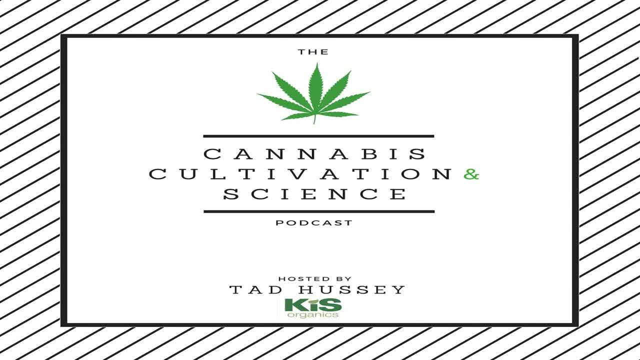 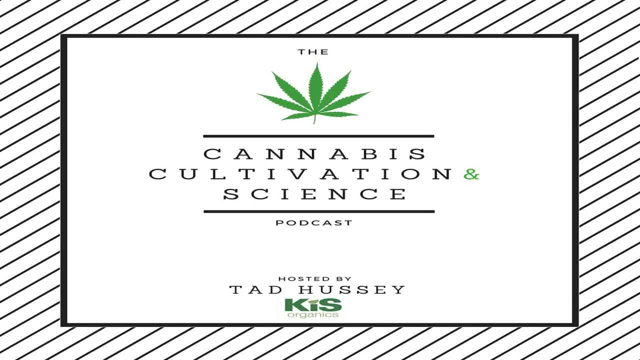 Yes, Yes, Yes, Yes, Yes. samples tested: That's a really, really good point And, from a statistical perspective, by increasing your end value- the number of samples that you're taking, I could probably take eight or nine samples for the price of what it would have cost me to go with the mass. 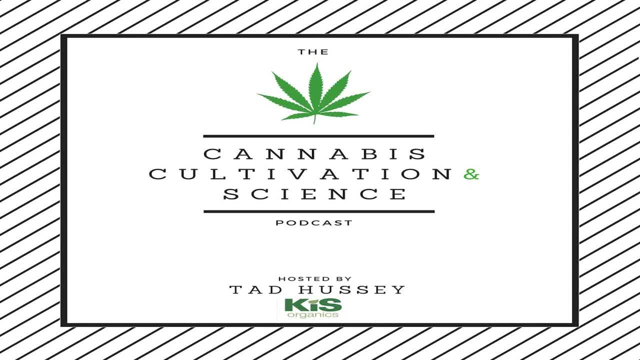 spectrometer. I can graph those and plot them and then come up with a more consistent value across all of those that would probably be as accurate or even more accurate of what's actually going on in my soil or in my fertilizer than you know one sample. So that's a really good point. you. 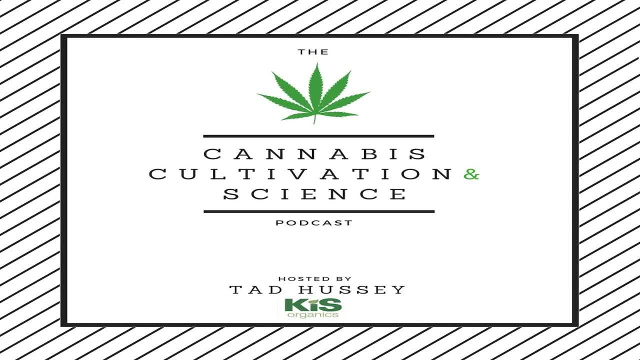 brought up there. Yeah, And this is something that the labs- university labs- I have noticed reading research, not just in the United States, but in some other countries as well- start using more and more this XRF method. It's their EPA or USDA method how to use? I think it's EPA. 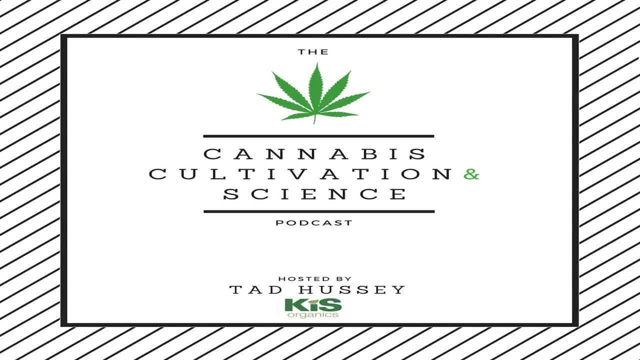 protocol. So it's developed to just follow the procedure- how to prepare a sample and analyze it, which also this machine also allows to test soil in a natural environment like outside. Of course, the result may be less accurate because it's moist or it's more heterogeneous. 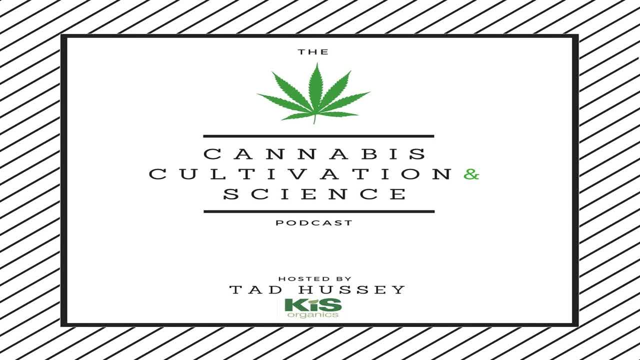 but still, if you go around the heat or even a garden, we can detect the hot spots of high levels of metals and collect those specific samples, And it's really good to understand variability in the garden or in the city like this is what I'm aiming to do in my research is 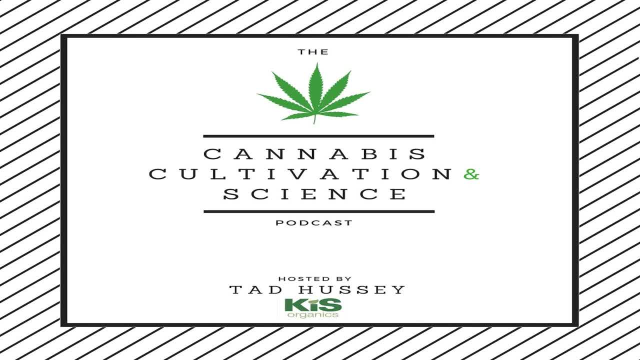 to analyze soil in Lafayette and see how metals are distributed here, And this instrument allows us to do it in a real-time setting. When we go around, we analyze it, we get the data within 90 seconds And then we can collect samples from highly contaminated areas and bring 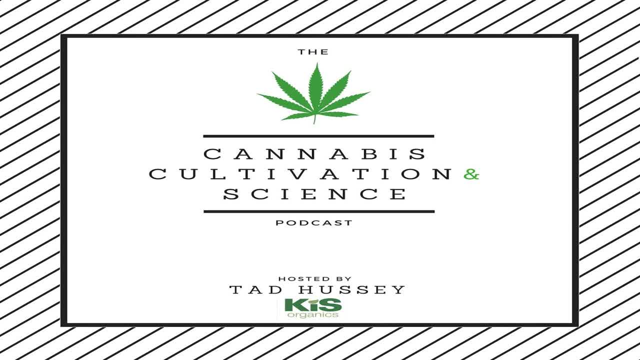 them to the lab for further, more accurate analysis. Now, in your research, how are you finding soil depth or compaction influences, heavy metals? Are the heavy metals more at the surface of the soil- Because I know you're talking about dust and things like that- Or are you finding? 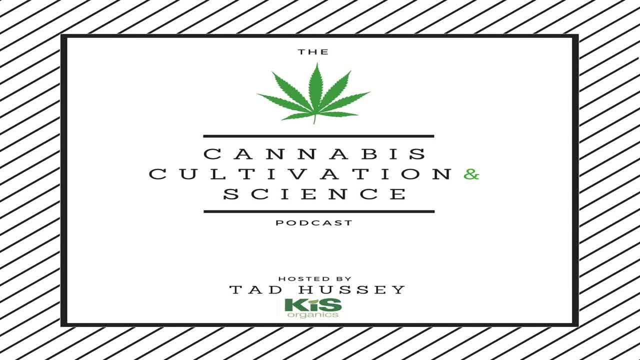 them further down, Like: could I grow a crop that's a deep rooting crop as a way of potentially helping remediate them, Or am I less likely to have contamination growing? you know something like a lettuce that's very low rooting? Yeah, so it's typically closer to topsoil or on top of the. 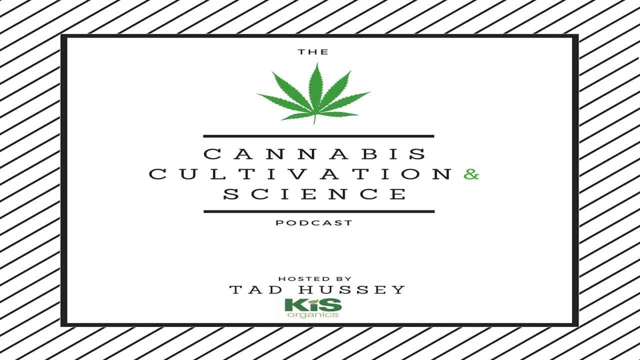 soil. If you don't add compost to your soil, just say it's normal soil. you will see it's closer to the surface or really like topsoil that most likely contaminated from all these deposits over the last I don't know. let's say 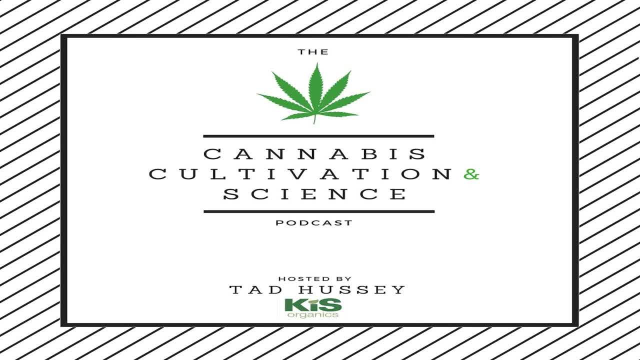 100 years that lead has been used or other metals been used and deposited from industrial sites, from highways, from lead paint. If you add something like your compost over and over every year, then of course you're burying your contaminants under, which is another remediation technique by the 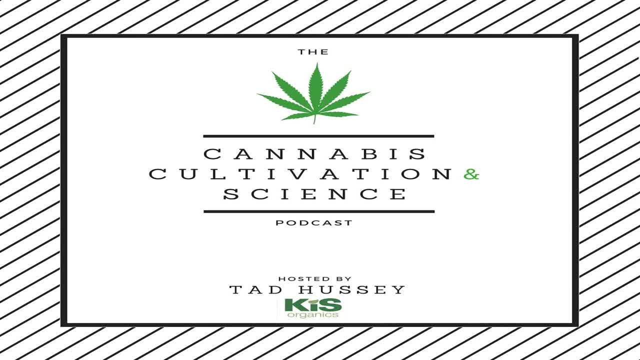 way. So yes, topsoil is most likely going to be contaminated surface soil, compared to topsoil, And dust and splashes is something to be concerned about. if soil is contaminated And if there are any children around, it's really important to make sure kids are not playing in. 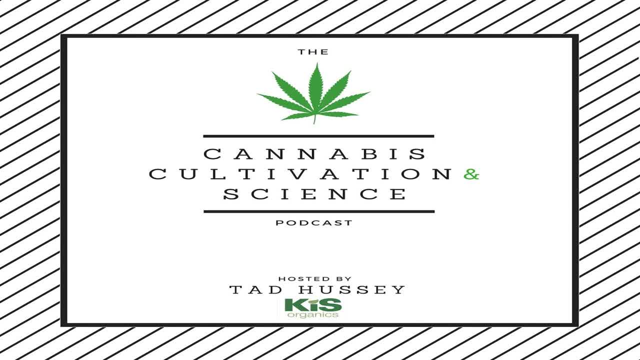 contaminated soil. That's a really good point. So, even if you don't plan on growing a crop, that's a really good point. So, even if you don't plan on growing vegetables, if you live in an urban environment, this would be a very simple way to just make sure that your yard is safe for your kids to play. 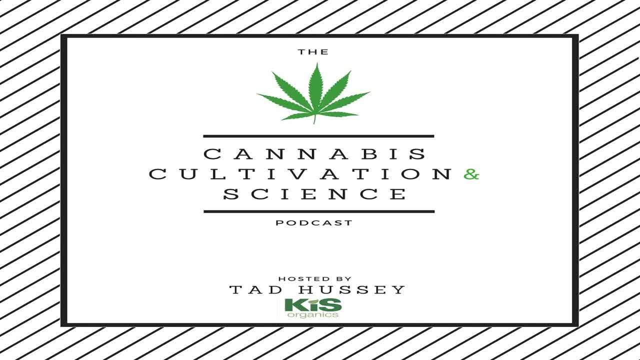 Yeah, it's even more important than for vegetables, because vegetables, as I said, like they pick it, they can. some of them can grow well and safely. some of them, like carrots, should not be grown in contaminated soil. But for children it's imperative to test soil the backyard to make sure the kids are not exposed, because the primary 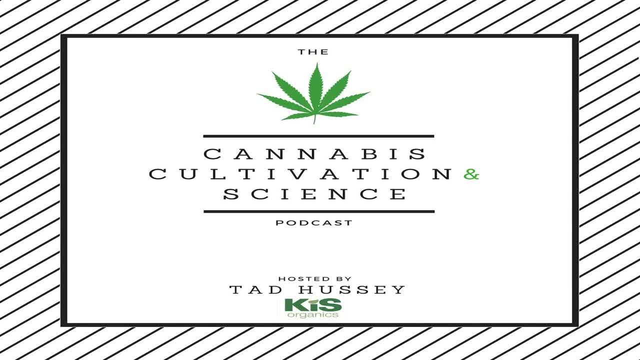 pathway of heavy metal exposure for people is actually ingestion and house dust. So children who are playing in the backyard on the bare soil: they would touch fingers and then lick their fingers ingesting potentially contaminated soil, And this should be avoided. And to do that, first test the soil, see what the levels you're getting and then plant some lawn on top or put some soil on top of it. 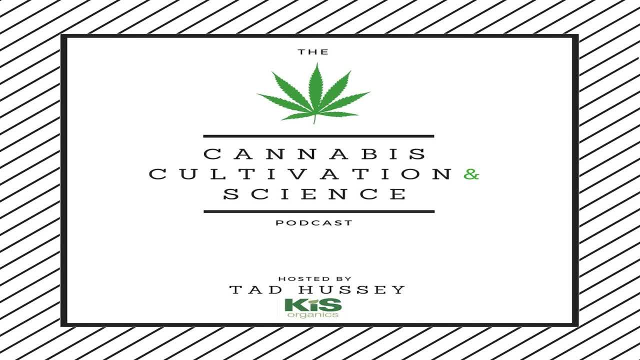 And then plant some lawn on top or put some soil on top of it, Some sort of fabric, some protection layer, so children are not exposed to bare soil. So definitely parents who have small children should test their soil just to prevent potential exposure. 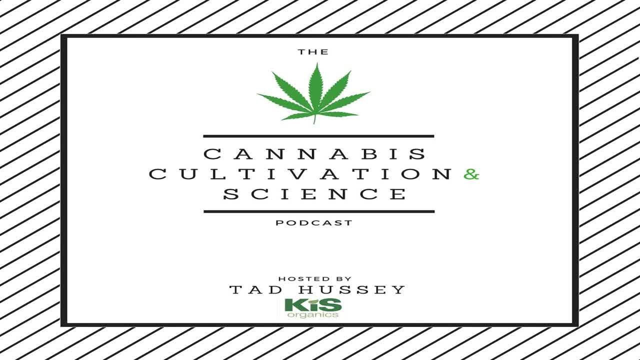 Yeah, that's a great point. I, as a new parent to a two year old, I am always thinking about this as someone who thinks about soil a lot, And right now we're living with my in-laws and they live on a golf course and I watch the chemical applications that are happening on the ground. 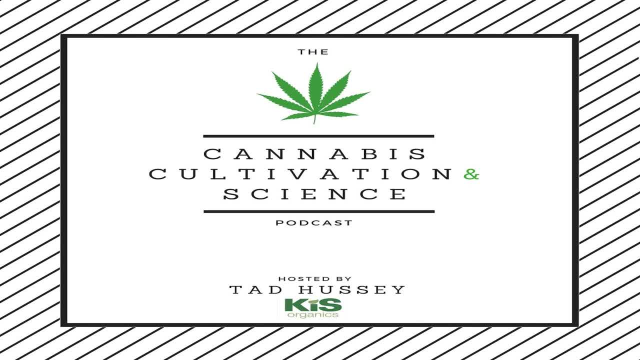 And I watch the chemical applications that are happening on the ground- And right now we're living with my in-laws and they live on a golf course- and I watch the chemical applications that are happening on the ground that have been contaminated. 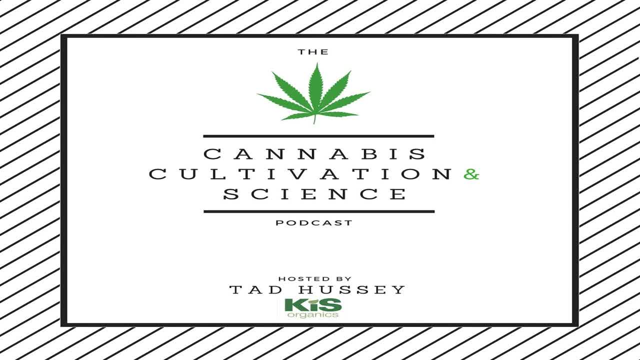 I'm thinking of Oklahoma just because I do a lot of work in Oklahoma and I know there's a lot of contamination sites there. So you know, parents, please do consider getting your soil tested And we'll list all the ways to, or the method to go about getting a hold of Anna. 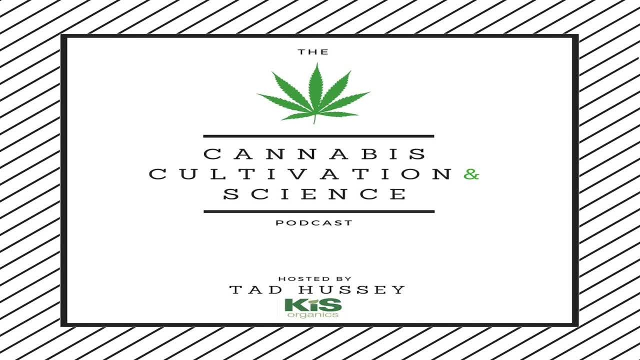 and submitting samples to her lab on the podcast page so people can get that information and absolutely get a hold of you for this. Of course, and we have also practices- how to remediate soil in case it's contaminated. I will share those resources as well. 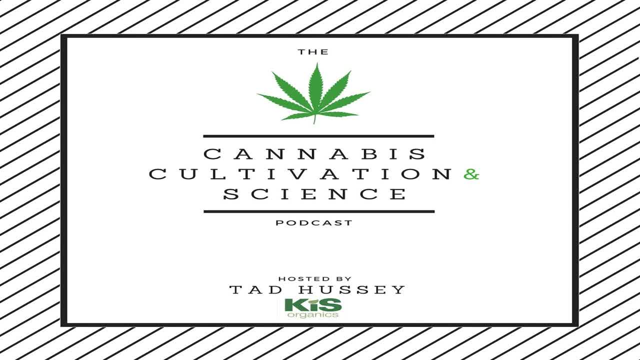 That was my next question. So let's say I send in my sample to you and whether I'm growing cannabis vegetables, I just want to protect my child and know the ground's safe. it comes back with high levels of arsenic or high levels of lead or cadmium. 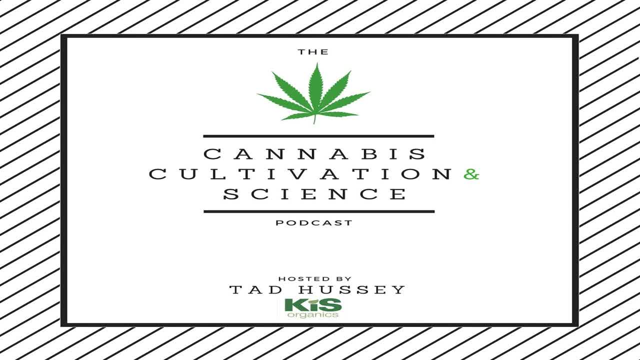 What do I do? Yeah, so it will depend on Now how high those levels are, but and where the how big the distribution is. it's a whole garden or just a vegetable plot. So some of the basic techniques to remediation is adding compost. 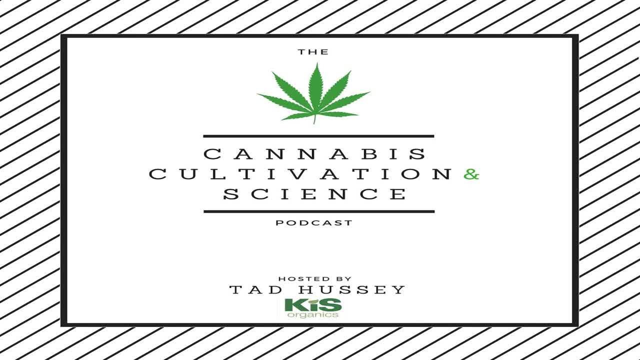 Or some sort of organic metal like mulch or something else that will help to dilute the soil And to bind metals with this organic matter. Another option is to put lawn on top Some sort of grasses to cover bare soil, So there is no dust. 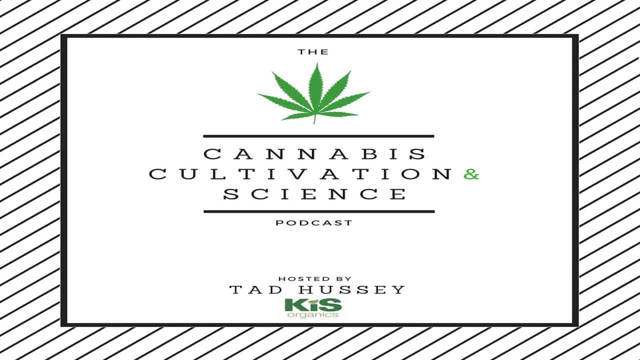 There is no erosion happening, reducing the potential runoff of the soil. We can plant in vegetation, add in compost or some sort of soil. You can try and change the chemistry of these metals by adding your phosphate ammendments or phosphate fertilizers. 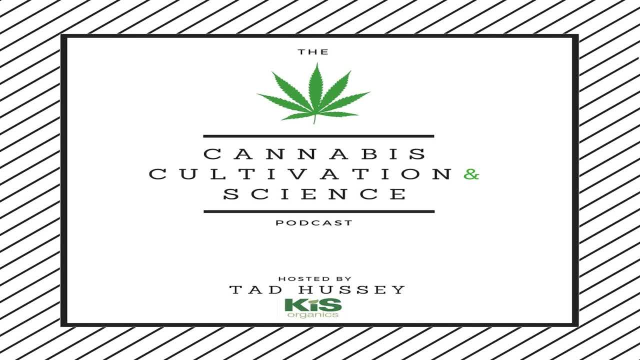 Although we found it would be tricky for an average person to figure out how much to add and how long it will take to break down, There are some studies that did a successful job with the change in your chemistry of lead and converting it to pyromorphic. 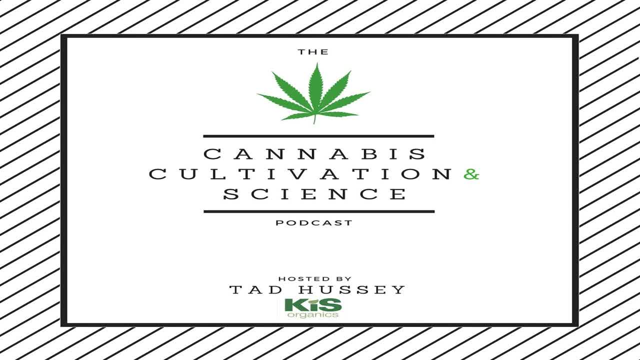 It's a stable lead-phosphate mineral, but for an average person it can be tricky to add And sometimes, if it's possible, you can bring a new soil, a new, cleaner sediment from some organic matter in it, of course, for nutrient content from another area. 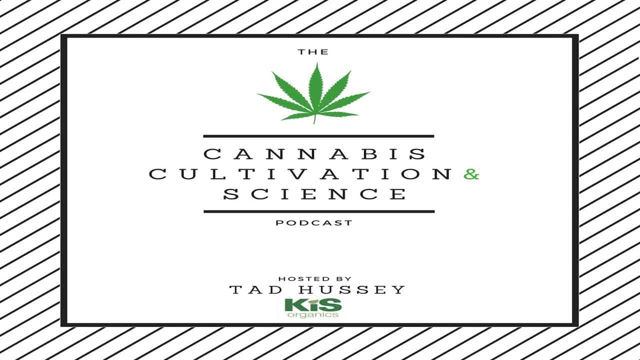 Some people take it from maybe like a farmland. Some people take it from maybe like a farmland. They know it's clean. or in New York, for example, there's a program that's called the Clean Soil Bank, when it actually distributes the glacier sediment to community organizations. 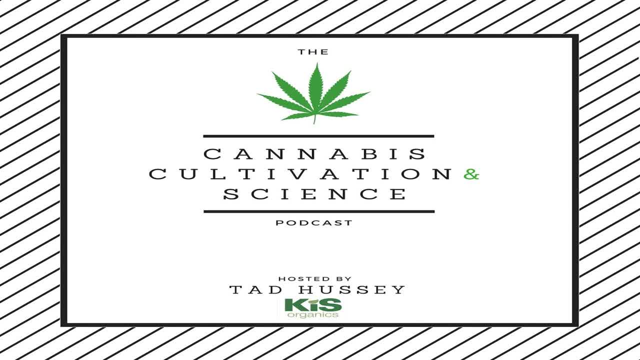 It's mostly sand, but it's clean, It's pristine because it was collected from deep layers when the foundation of a new building is being constructed. And that glacier sediment in the community. And that glacier sediment in the community. And that glacier sediment in the community. 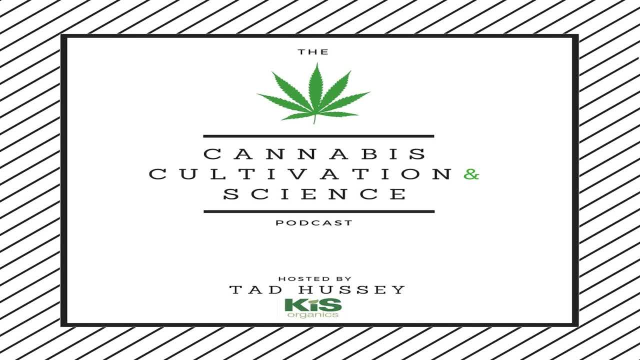 garden, let's say, can be mixed with the compost to provide nutrition value and successful plants can grow and of course, it's much, much safer for children. so if there is a way to bring a new soil, it's a possibility using raised bed soil or build a raised bed on top of contaminated soil. 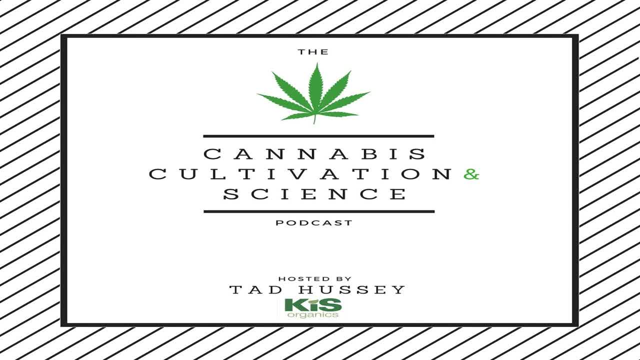 it's an option. if you don't worry about children, if you don't have small kids and you only want to grow vegetables and you don't want to do any amendments or any compost additions, then grow tomatoes. they found to be at the model. you can grown well in the moderately contaminated soils. 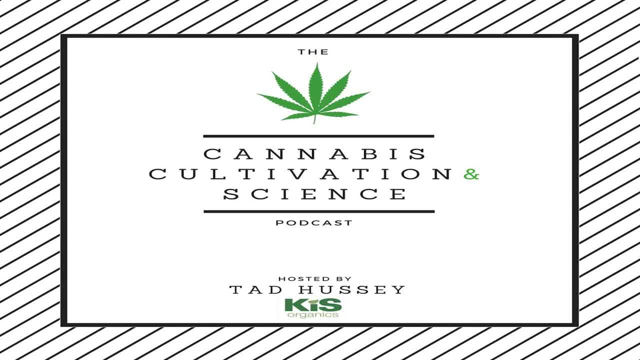 because they have physiological barriers inside of them that prevent metals to be up, taken to food and that, further from the surface, that told plants and they don't really have splash, it's from surrounding areas. so those will be very simple techniques, probably least expensive. of course you can excavate it and bring absolutely new soil, but it will be more expensive. so so we've. 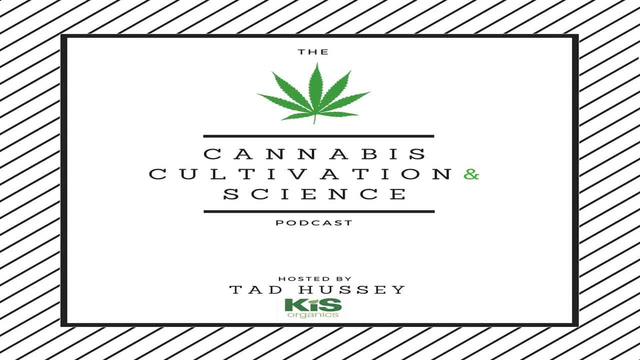 been talking about soil as the primary source of contamination, but can we talk a little bit about where this is all coming from? it's not like that soil started out contaminated where. where is this contamination coming from and how do we limit that in? you know, not just our. 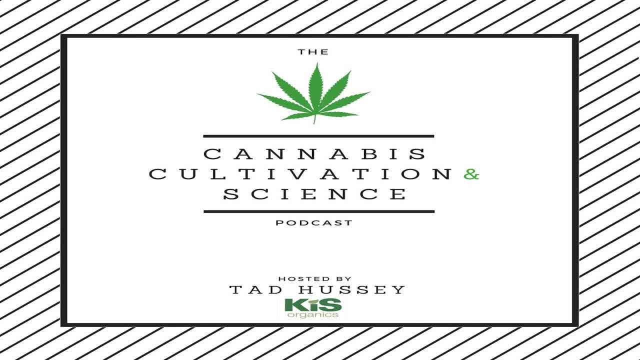 gardens, but also our homes. uh, good, good question. so one thing to know that the metals naturally occur in soil from parent material such as rocks and minerals, but those levels are typically very low and they're not harmful to people because they're natural sources. however, we do have 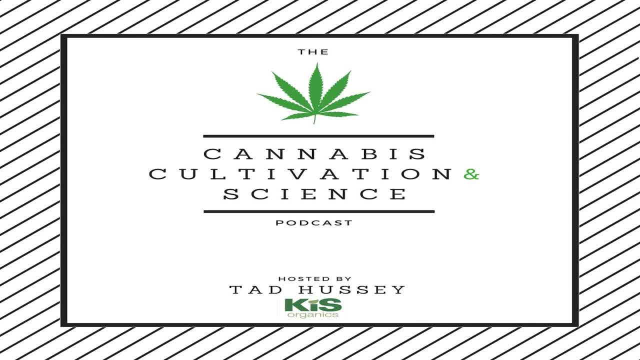 organic sources of metals, which in most cases is industrial sites. it's uh roads, cars, vehicles and uh paint- leaded paint. of course. it has been banned since 1978, but lead paint is still on some old houses, so it's important for people to know what kind of paint they have on houses, if they believe. 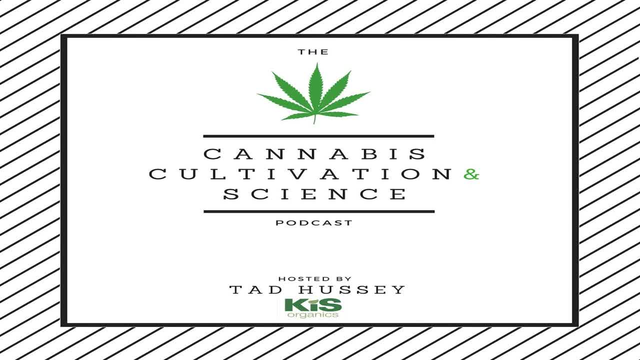 in them and they know they have before 1970, so the most likely will have some lead. so it's really important to know that part and then do testing of surrounding areas if possible. you can even test paint chips these days as well. so it's important to reduce the house dust, so especially if there are children in the house. 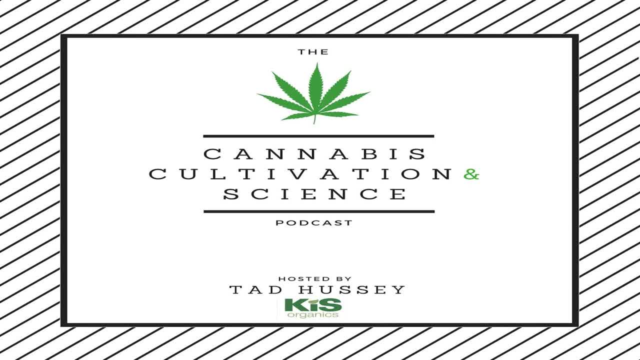 by doing your cleaning, just like, you know, with a some wet napkin or something, so that so they could down the dust. dust is one of the main sources inside of the house and this dust can come from, uh, you know, from windows, from open doors, from shoes that people work outside or walk outside. 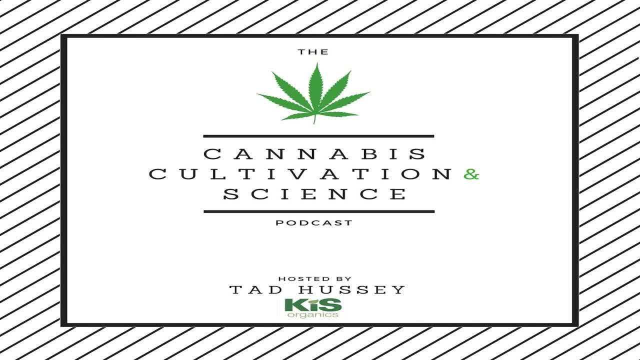 and bring this dust, dirt into the house. so, to avoid this, leave shoes outside or change shoes when you walk inside. don't bring dirty instruments from the garden of the house and do wet cleaning like wash floors and wash window ceilings, uh. so yeah, those are basic recommendations, uh, to reduce contamination inside of the houses. 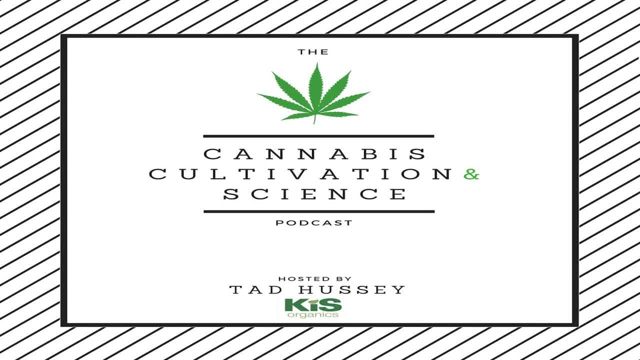 um, we cannot change land. you'd use history of locations where we live because you know they had some industry industrial sites in the past. but we can uh control our environment inside of our homes by just doing good cleaning medically and testing uh what um surrounding our houses and knowing the history of the house or at 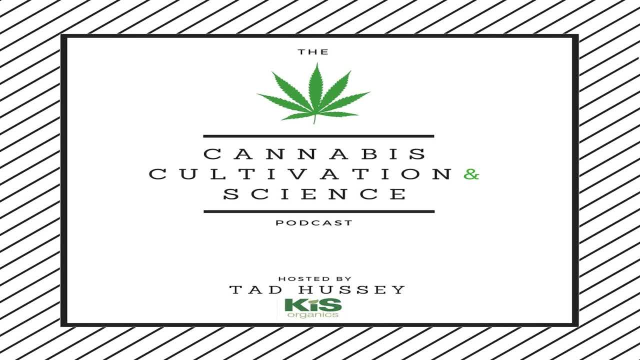 least when it was built. that's it. that's a good point. and one other thing, people, I want people to consider when we're talking about edible crops and food crops is everything that those roots or that soil is coming in contact with. so if you're going to build a garden, think about the material. 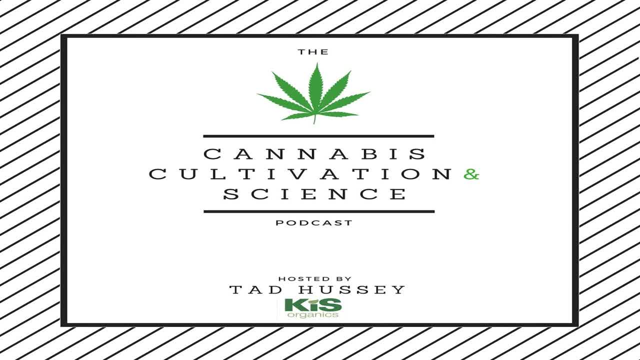 that you're using to build with- yeah, even with- fabric pots. I've saw some research, um, some pots coming out of China that showed high levels of lead. so when those roots hit that edge of fabric, that fabric pot, they're being exposed to that lead and they could potentially 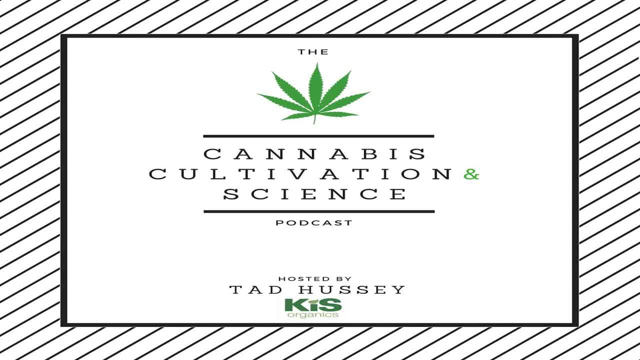 be taking it up. so, um, there's just a lot of things. you have to really think like a scientist or like a detective when you start thinking about labels too. yes, yes, so, um, well, great, I want to kind of change directions here. um, we've been talking about heavy metals related to gardening and urban soils. 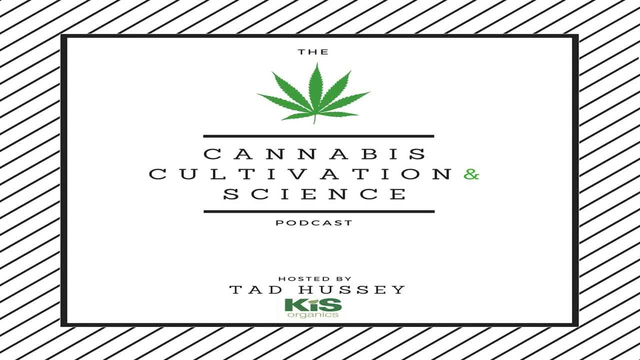 um, since this is a cannabis cultivation podcast, um- and I know your experience is not with cannabis, I I wanted to talk a little bit about, um, heavy metals, that you know some of the how that might relate to cannabis and get your thoughts on some of this. so one of the things is, in certain states, 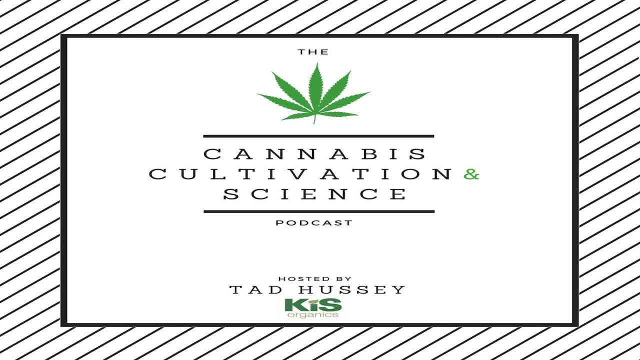 now they're testing the flower for arsenic, cadmium and lead and a fairly aggressive thresholds and it appears to be, uh, a fairly good at uptaking not just nutrients but these heavy metals, and we are seeing some failures in certain states based on the methodology that people are using. 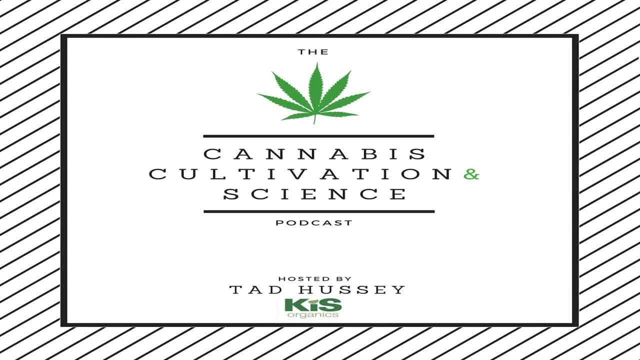 um, you've already talked about ways to sort of reduce heavy metal exposure. um, you know we're not testing vegetables like this. do you think that down the road policies might change in terms of how? how we're testing, like maybe cannabis, might be sort of an example for how we may eventually test vegetables? 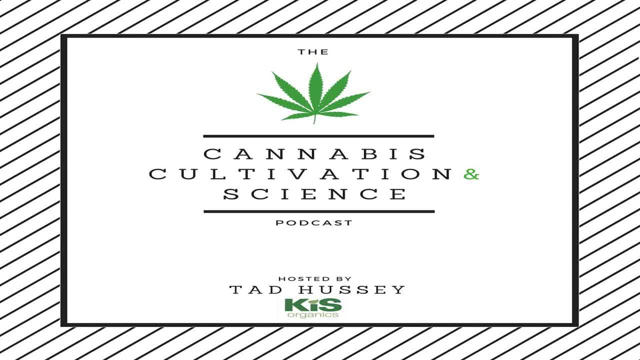 that's a very interesting question. I think of part of the answer here would be to understand that cannabis is not a simple plant. it's hyper accumulator plant and that plant, basically, is capable of uptaking metals from soil, and I think this is why policies really forcing on measuring cannabis- not so all vegetables have. 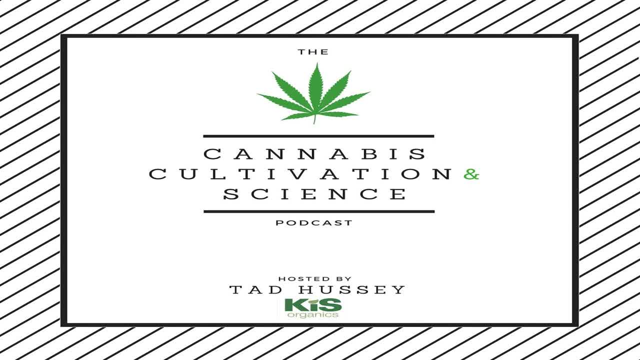 taken up metals at the same level. so each vegetable of food or berry or tree versus grass, they have their own capabilities, how much they can or willing even to uptake metals and how they tolerate it. some can be more susceptible than others. some plants may be affected by even low toxicity levels. others can be much higher. some of them we 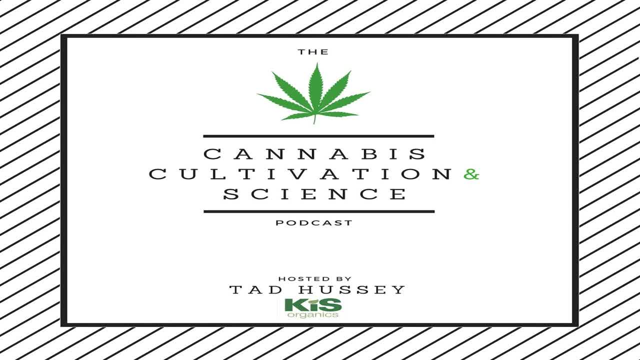 prevent contaminants going into their tissues, like tomatoes. so there's no need as much as cannabis to test tomato plants. so it's really important to understand what type of plant that is and when it comes to hyper chemical plants or plants that we know can take more metals than the average. 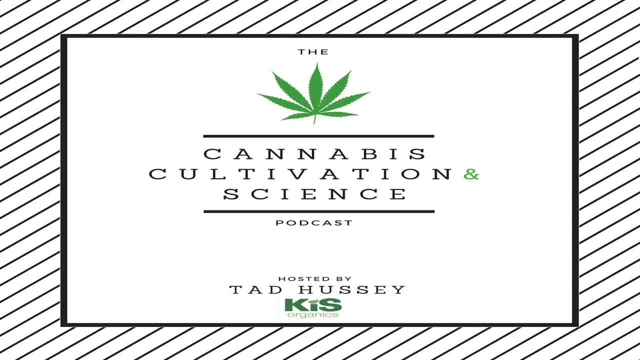 plants, then it needs to be more vigorously regulated. so I'm not the policy person but like from a science point of view, that's how I see it. I I mean, I would love to see, I would love to go to the grocery store and eventually have there be, you know, conventionally grown, organically grown, heavy. 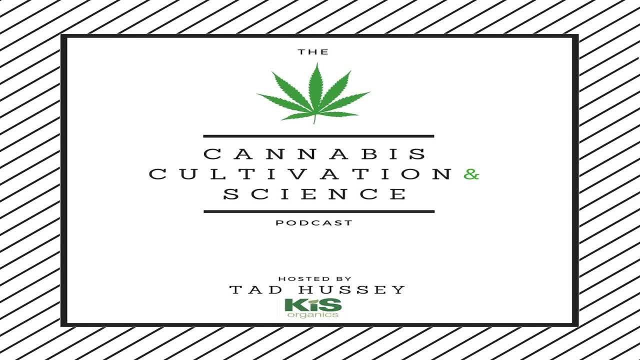 metal free. you know half of some of these new labels that would allow me to make choices, because I would pay a little bit more to know that what I'm buying is is free of of certain contaminants beyond. you know, just the organic certification, um, but who knows, that's a great point and I, um, yeah, I don't know the answer to. 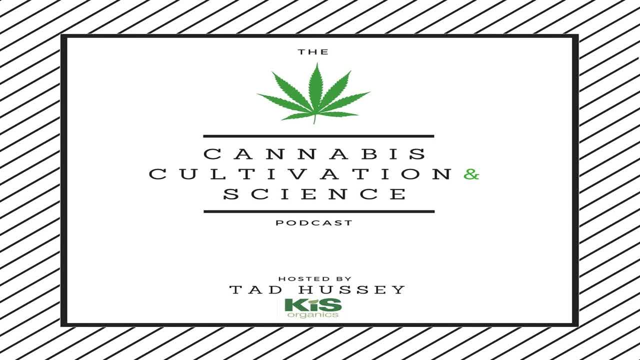 the question, but I think it's definitely more interesting. and it comes back to uh testing and pricing for testing, right, because if we have to test everything, everything, then every batch it will be lots of data, a lot of processing, a lot of labs and a lot of delays, uh, but I think 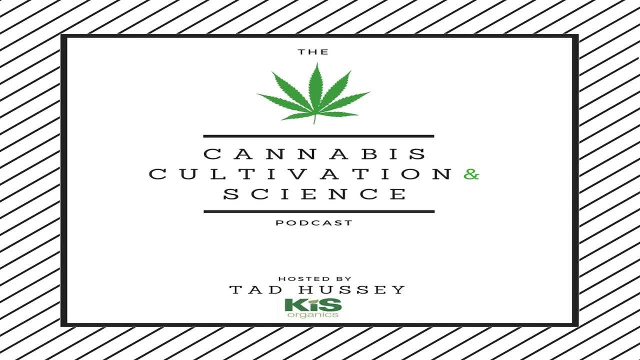 having more vigorous food. uh testing is good and I know FAO recently was bringing it up that they were collecting data from scientists around the world on uh- I think it was mercury and fish. they would want you to see more data on it. so I think it is moving towards uh food safety testing and 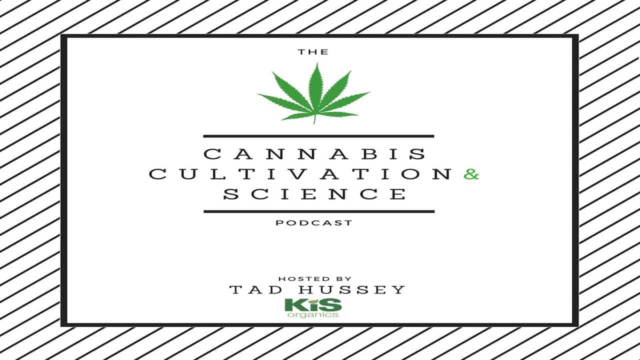 metals and perhaps other contaminants as well. but it's you know it takes some time to be able to do everything. so can I share with you some of what I've found in in cannabis, um related to heavy metals, and please just correct me if anything I find seems, say, seems odd or wrong or inaccurate. 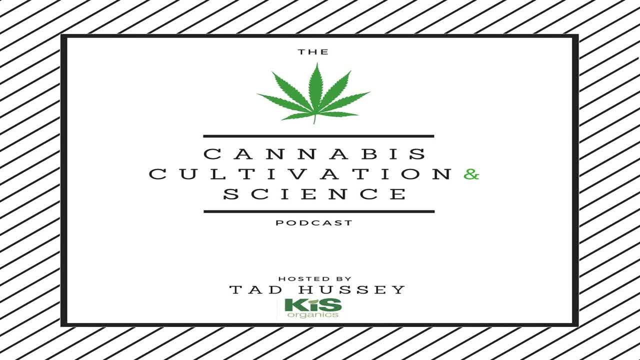 um, but since, since we've been, we've been diving more and more into this, this heavy metal thing, because, um, we've had a few growers fail and you know, as someone who manufactures soil, in addition to this podcast, um, and and the fact that we do organic soil and organic amendments, uh, you know, there is always going to. 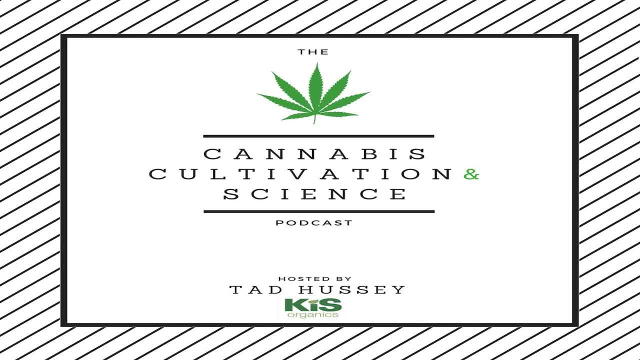 be some heavy metal load in our soil, and so we're always looking at how to reduce this, because we use things like rock dust which, as you know, contains levels of heavy metals and soft rock phosphate. um, you know, any mind product or um, in my experience, contains some level of heavy metal. 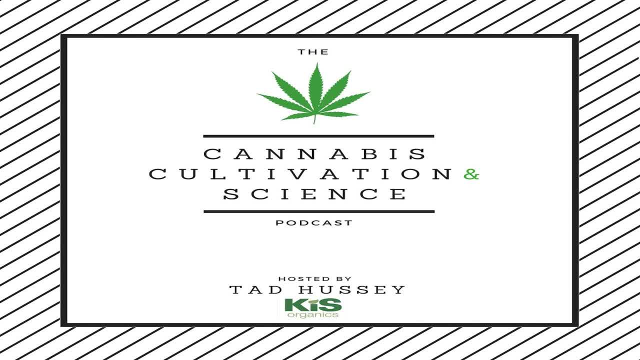 so it's all about heavy metal management. we can't reduce it to zero, but we want to make sure we're not overloading it. and then um, beyond that, keeping our pH a little more alkaline. so I like to run my pH higher than traditional um agronomic recommendations, um probably closer. 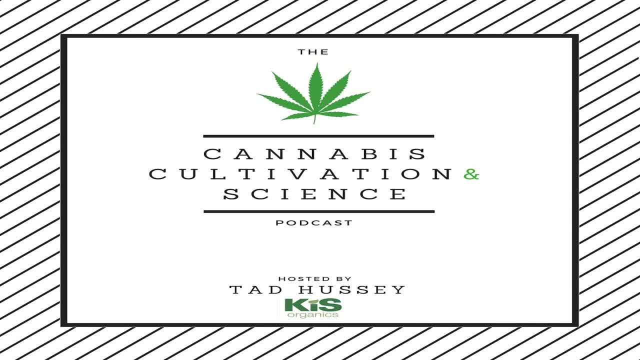 six, eight to seven range, rather than, you know, six, four, six, five, like I see, like I see in a lot of places. um is sort of the sweet spot for me in terms of heavy, in terms of reducing heavy metal risk but still allowing for good nutrient availability, um in terms of exposure. so, um, you know, I just want. 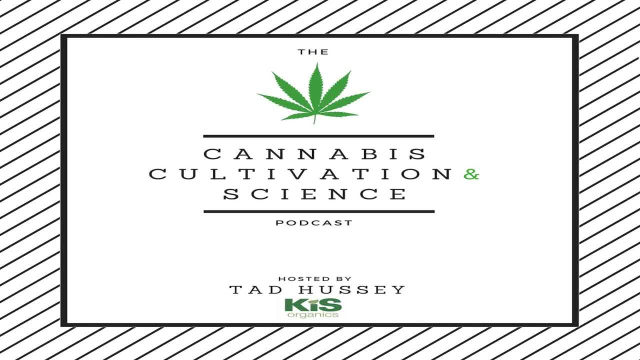 to throw out there. no one's failed just using our soils. we've always found other sources of contamination that were more significant and really contributing to a fill rate. um, some of these were water sources. people thought they had clean water, but they were from a well and 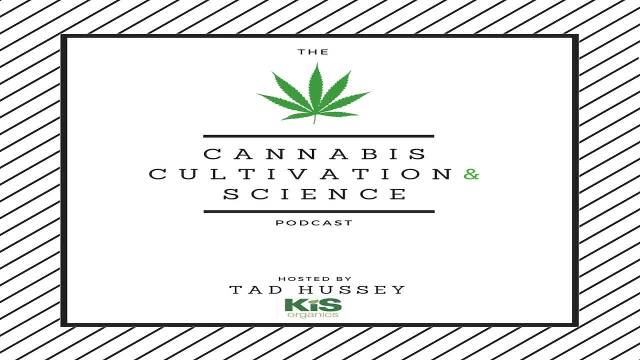 they actually were bringing up um groundwater- in this case it was arsenic um. I had another one in the facility. that was an old building in Oklahoma City and they were doing a lot of construction and they were kicking up dust and that dust was falling onto the leaves and causing contamination. 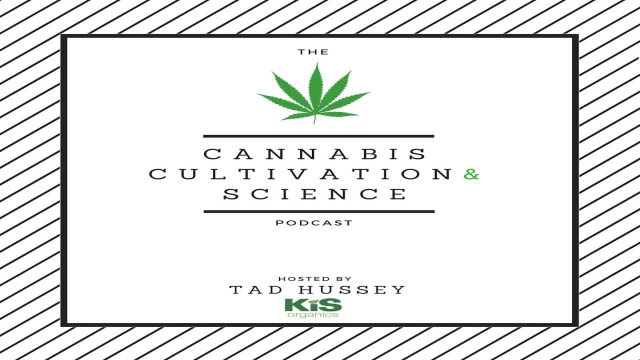 um, so that was a little bit of a tricky one to figure out. even things like, uh, sump pumps or metals that are in contact with water for a long time, like in a reservoir or through an irrigation system, we found can increase a heavy metal load too. 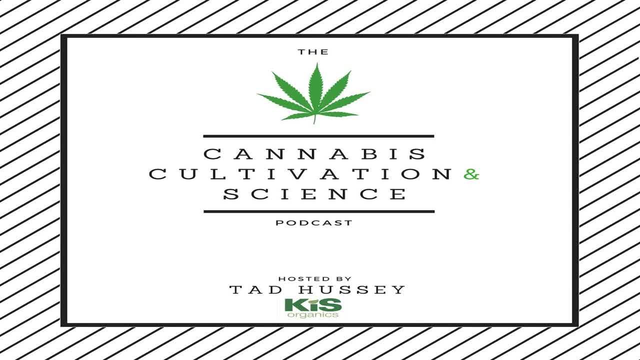 um. so it's, it's, it's a challenge and you're always trying to figure out what it is. and then um I I guess one thing you brought up was phosphates, which I thought was really interesting, and how they might bind up um lead. you know, one of the things that we find with um. I've been trying to. 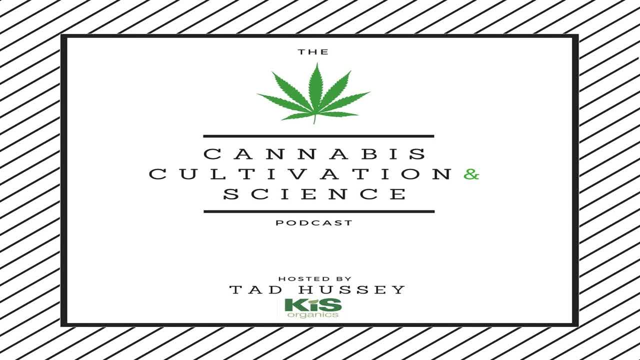 find a good phosphorus source that was uh vegan or not animal based, and it's it's really really hard um. all the ones I find are also, um bringing in uh heavy metals. I sent one sample to you of a soft rock phosphate and it came back. 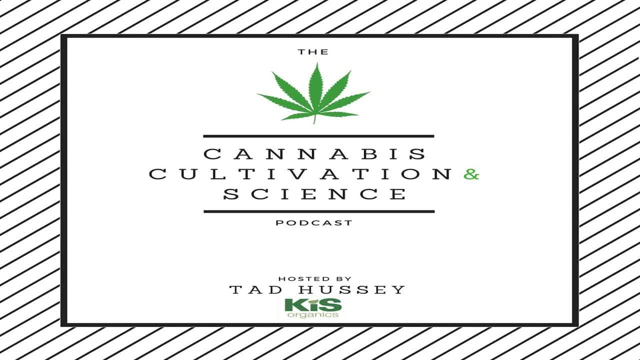 with. you know lead levels, so how one do you know of any great phosphate sources that are going to be lower in heavy metals? and then, um, can you talk a little bit more about this phosphate binding? yeah, oh so, yeah, that's a good question. on sources, one thing that came to my mind is the: 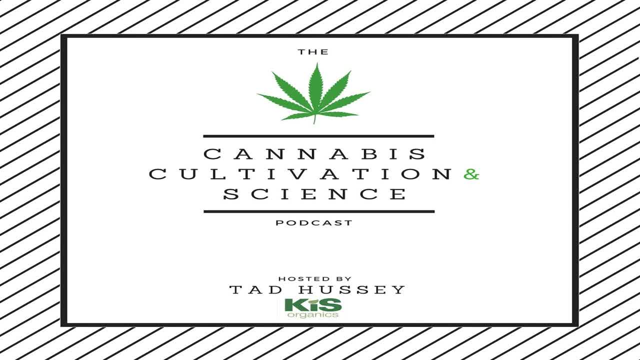 uh, fish bones, but it's not. I mean, you said, uh, you wanted it to be vegan or like not animal products, but then, yeah, it's appetite. uh, it's a traditional, uh rock mining, you know mineral which is running out, so we need looking, uh, look for other phosphate um sources, but yeah, fish bones would be. 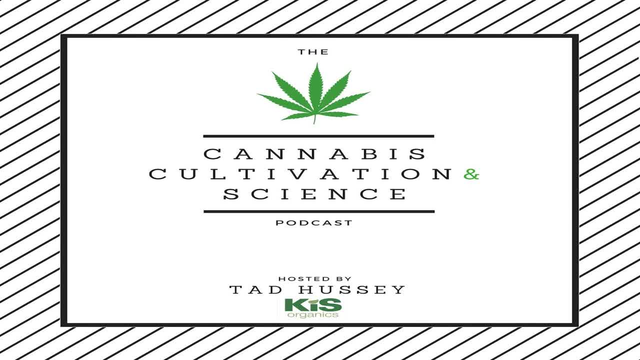 non-vegan uh source which might not have as much heavy metals as anything else? um, otherwise, I don't know. it's it's hard to think. um, I have to think about this one and get back to you if I find the resources. yeah, it's um, typically fungi would help to release phosphorus. that's in. 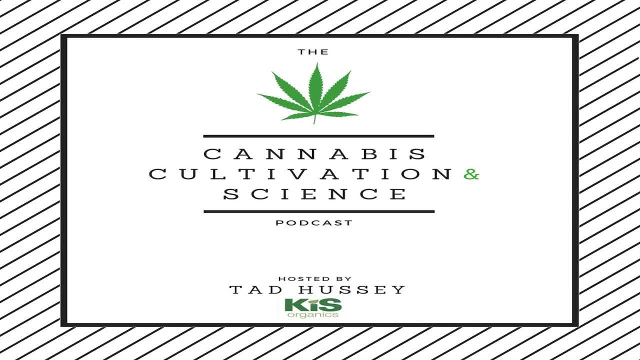 the environment, making it more accessible for plant uptake. so maybe there will be some mixing with fungi that could be. now I developed more uh uh. Dr Allison Justice actually sent me a paper a couple of years ago out of Italy that showed uh with hemp increased heavy metal uptake into the hemp biomass with the addition of 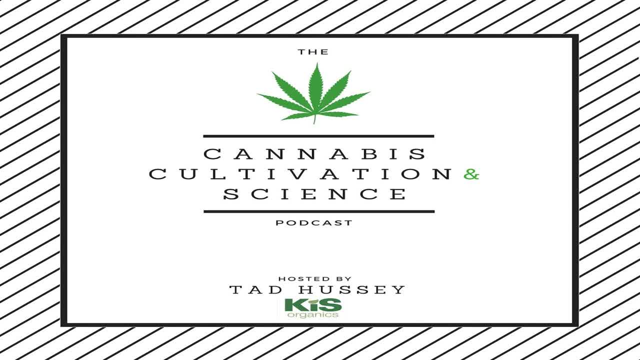 mycorrhizal fungus, which makes sense to me, because mycorrhizal fungus increases the uh nutrient uptake. you know it's most notably phosphorus, but um other nutrients as well, and so they saw higher levels of arsenic with um uptake with it, which which i just thought was. 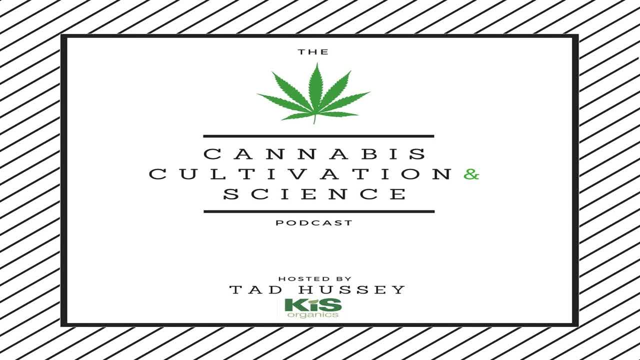 interesting research. um, so i i guess maybe my question: arsenic becomes more. arsenic becomes more available with phosphorus addition, while lead becomes less available with phosphorus addition. so that's a paradox when both lead and arsenic are present in the soil. i didn't know that's. 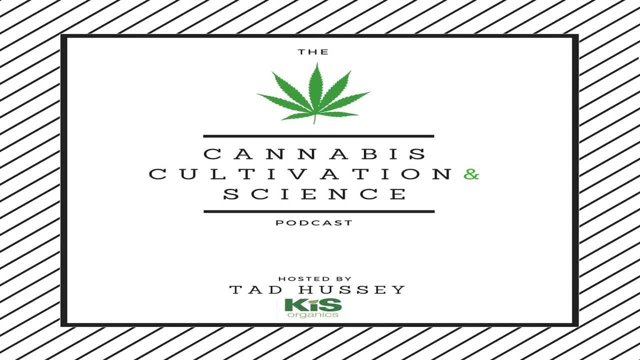 all. phosphorus might not be. yeah, so phosphorus might not be the best solution if soil is contaminated with both lead and arsenic. when we did a test for heavy metals in our research in new jersey, we tested the soil that was contaminated with lead and arsenic. 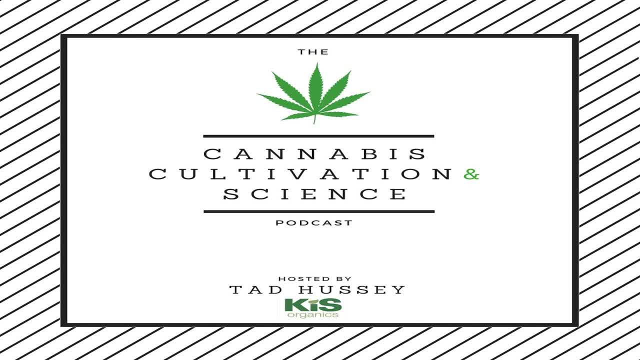 and we added the different phosphorus fertilizers and we added different compost and we saw that arsenic was more available, did not, was not fixed by phosphorus, obviously, because they start uh competing and arsenic becomes more mobilized- but compost was a better result for us. 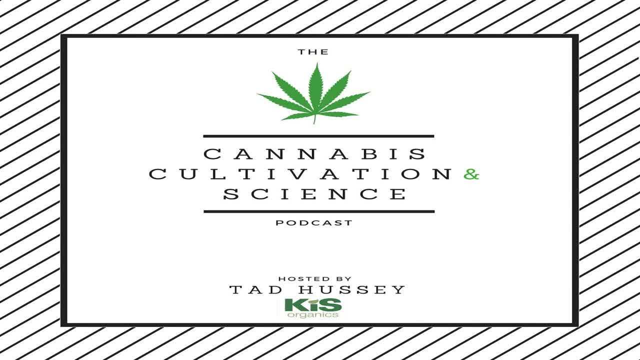 and showed the basically, yeah, it was more successful as a remediation technique compared to phosphorus fertilizers. that's. that's really interesting. um now, one thing you mentioned was that arsenic is more leachable than lead. how realistic is it for someone to flush their soil or their their, their media as a way of reducing arsenic levels? is that going to? 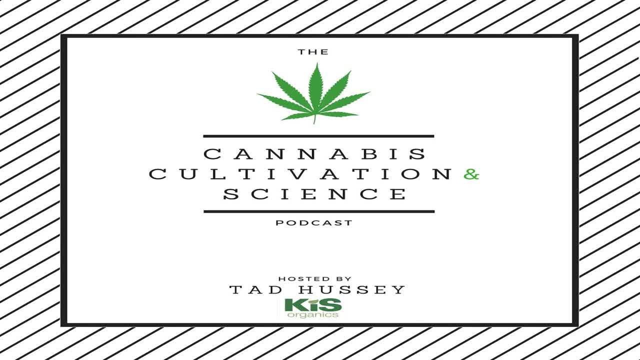 make a significant difference. oh, that's an interesting question that i'm not capable to answer fully, because i know there is such thing as an industrial washing, when, like you know, they do it on a large scale and they can wash soil, uh, with water or maybe some other solvent. that 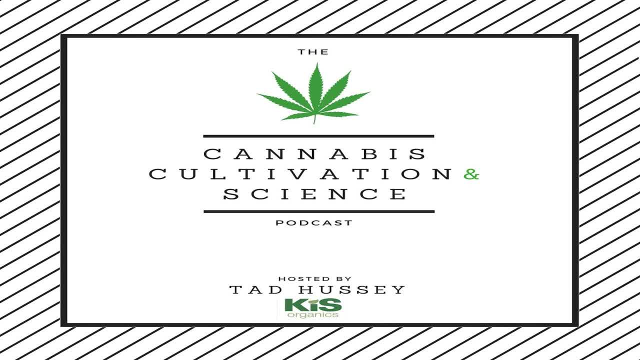 helps to remove, uh, heavy metals, but i don't know for if it's sufficient for a person to do it. it's just not something i've seen in literature because i've never was curious about it until now. that's fair. i i appreciate your honest response, but i am gonna tell you i'm just very glad to hear about your answer and i hope you enjoyed this talk with me and i'll see you guys next week. Bye, bye. 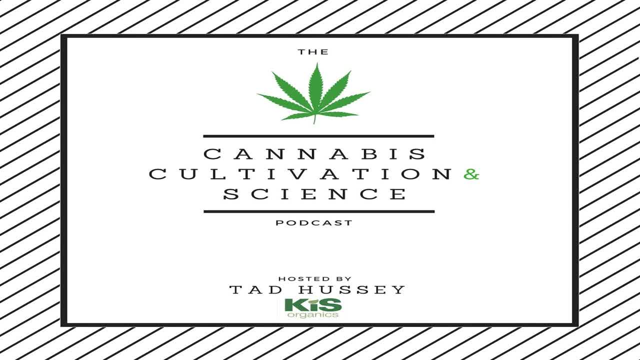 I would think it's not super leachable just because we still see it in areas that have fairly significant rainfall, Right, If there was, you know exactly precipitation and nature, yeah. So they maybe needed some technologies to do that. yeah, to make it more effective. 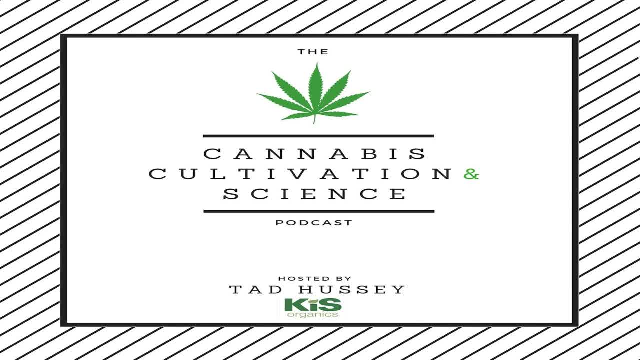 If it was like nitrates, for example, then we would know pretty quickly it would just disappear into our water. Yeah, I wonder if there's a microbe down the road that someone will discover that will allow us to tie up these heavy metals more efficiently. 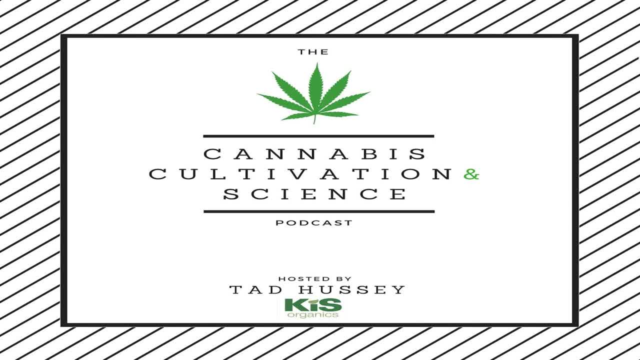 That would be a really cool invention or discovery. I guess we would say Yeah, I think there are research studies related to that And it was promising to find some microbes that are converting metals into less available forms, And also fungi help to convert lead to paramorphic. 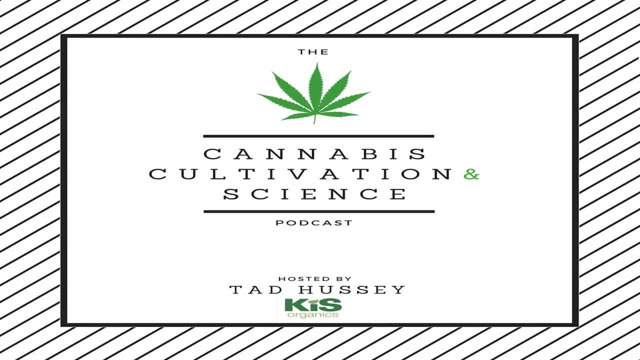 And you asked me earlier about this conversion. So what basically happens is, when lead is exposed to available phosphorus, it combines into paramorphic. But you would need lots of phosphorus in the environment to combine this lead efficiently And it will take some time, sometimes maybe a few years. 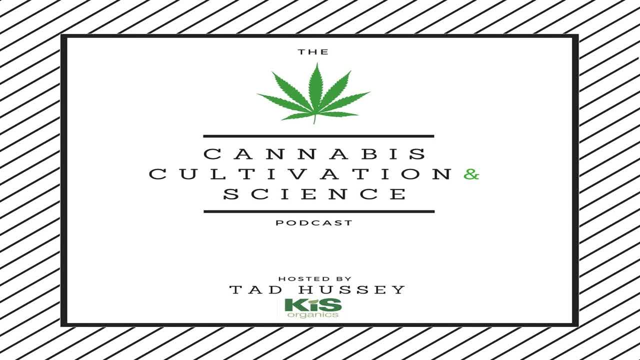 It depends on the climate, It depends on the zone where the site is located, But the idea here is that just lead becomes lead phosphate mineral And it's very stable And it's not bioaccessible or has very low bioaccessibility, So it's not really harmful to people. 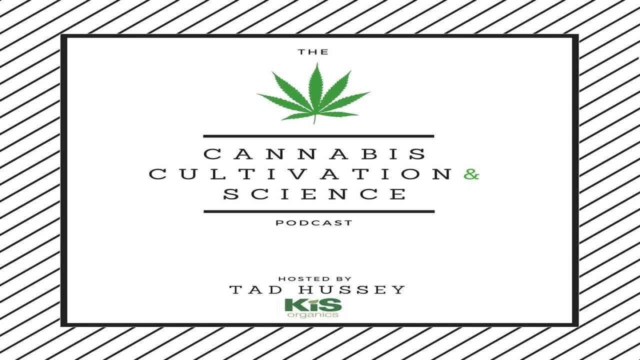 If it gets to human body, like, let's say, a child consumes it, it will just go through the system And you know, just the child poops it out. But it's not being dissolved in a bloodstream, compared to other forms of lead. 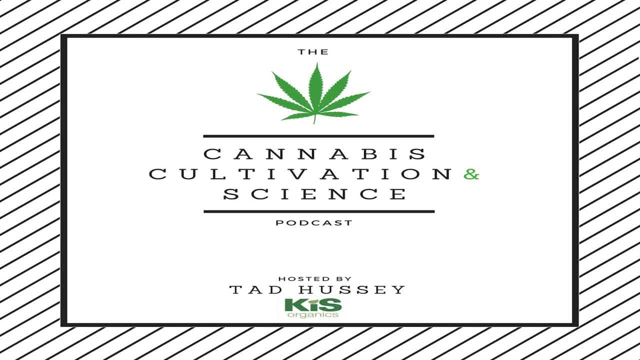 So paramorphic is a really good mineral to have, But it takes time naturally to form it or artificially to form it If you want to play around in your garden and try to make this conversion yourself. So when we get a lab test back, that's not going to tell us the actual. 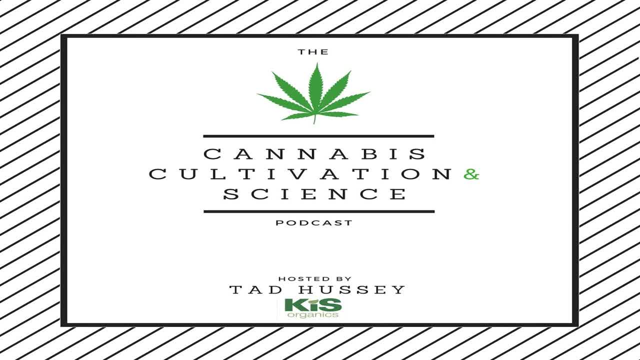 Form of the arsenic or the lead. So we won't know how available this is to our plant. We'll just know that it's present in some form. So good question. There are different methods how it's tested. Metals can be measured in total concentrations and phytoavailable concentrations for plants. 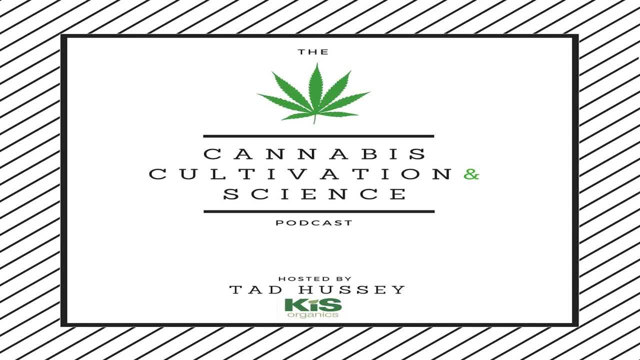 And in bioaccessible concentrations, Total concentrations. It just gives us total numbers of how much in total lead or arsenic or cadmium in soil Phytoavailable. those methods are using extractions to see how much potentially can be uptaken by plants. 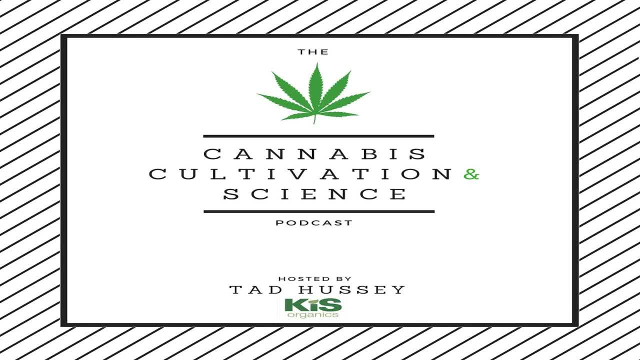 Or how much is available, at least for a plant, And it will be lower than total concentration. typically, Not all of it is going to be available. This can be found in labs, A lot of labs testing for phytoavailable nutrients, but also metals. 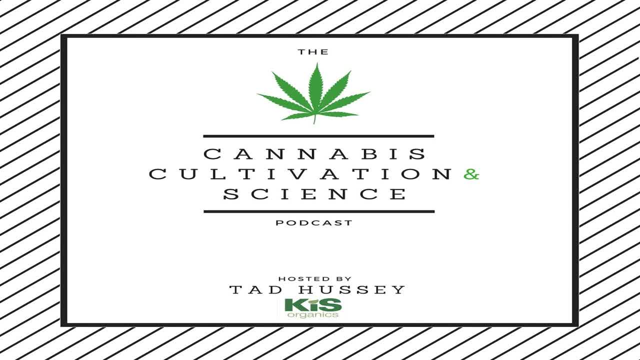 And another question is bioaccessibility. I've seen only a few labs around the country who test for that for public. It takes more effort to do that method and do sample preparation And the method is still. there are different methods how to use it. 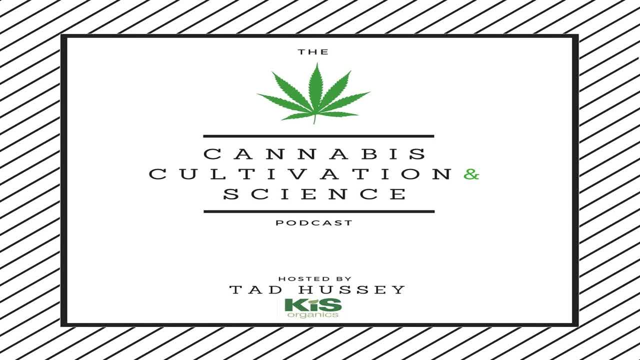 There's an EPA method, there's a European method. different authors came up with a different method, So it's hard to say which one is the best. and it's still tricky in some ways to assess the bioaccessibility, Because when we do these extractions we try to mimic gastric solution in the lab condition. And it's really difficult to predict what is the human gastric system is and you know like our chemistry of gastric solution changes if, like before we eat, after we eat it will respond differently, potentially on the metals we would consume. 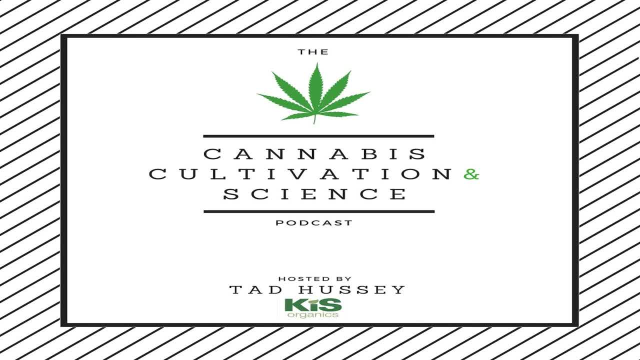 And it's very difficult to mimic this in the lab conditions. That's why there are so many methods that exist out there And the labs don't- really not many labs offer those tests. If you get the chance to find a lab that tests for bioaccessibility, you should do at least several samples for you to get an idea what numbers you're getting. 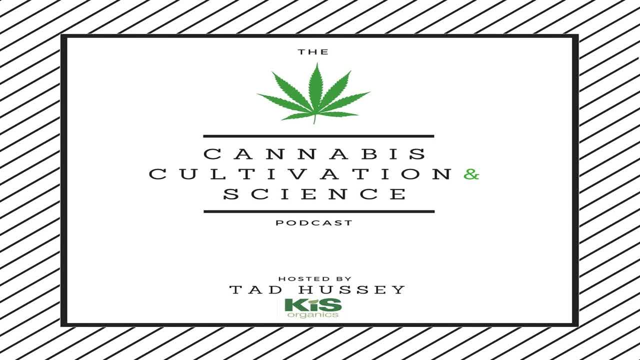 Okay, so it's not very cost-effective, necessarily, or realistic for the average person or grower to find that out at this point. Yeah, I don't know the prices. Yeah, I don't know if they're like, what are the prices for them? 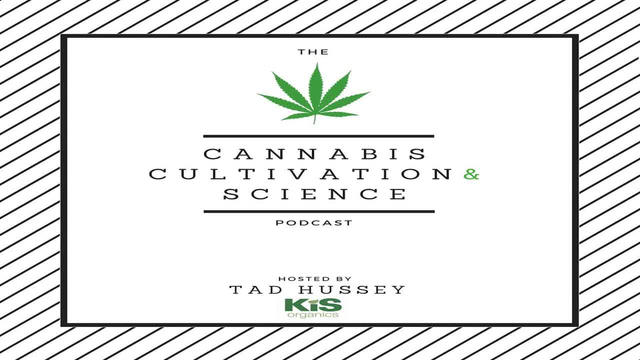 They're just not as publicly available. Yeah, I don't know how publicly available tests, as I've seen, Like not every laboratory offers that, Okay, okay, And while you were talking about that, it got me thinking about one other variable that I meant to mention that we've kind of touched on is not just crop selection in terms of variety, but also or species, but also cultivar selection. 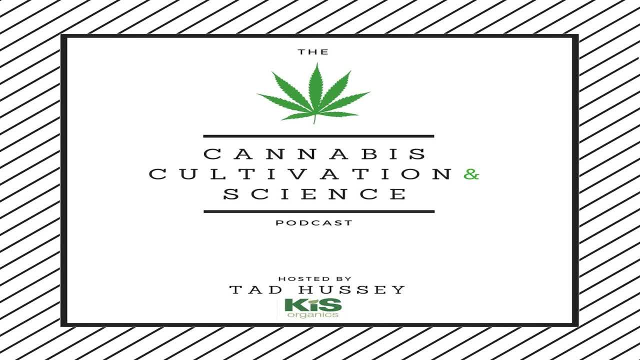 So the amount of genetic diversity we see in different species, Yeah, Yeah, That's a really good point, And I think the amount of diversity in cannabis is huge. It's much larger than any other you know ornament or vegetable crop that anyone would grow. 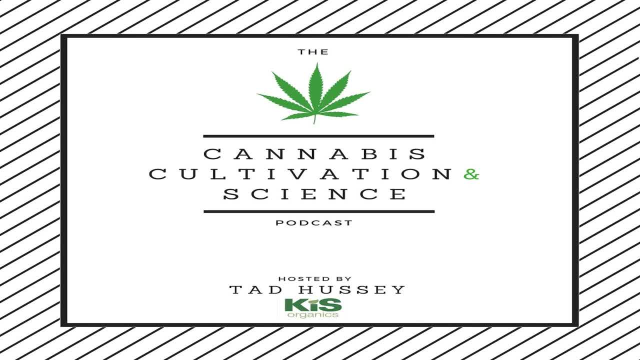 So we found that certain genetics will uptake heavy metals much more efficiently than others. So just because one genetic fails, doesn't mean that other ones will fail in that same soil. So that's just one other factor. I mean, there's so many variables here when it comes to heavy metal uptake that you've touched on. 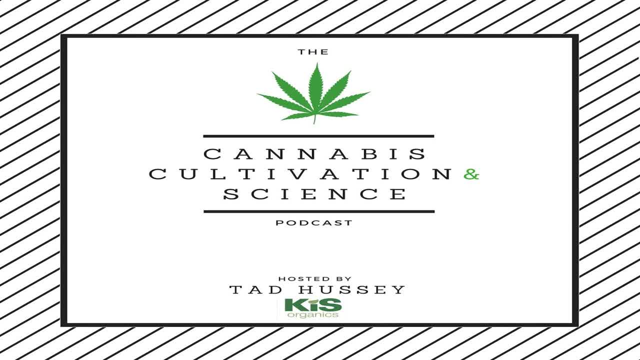 It's just. it's a complicated topic And I'm sure there's more to learn in the future. Yes, yes, It is, It's complicated. Yes, So is there anything else that you would like to share before we sign off, in regards to your research or upcoming research, that you're really excited about? 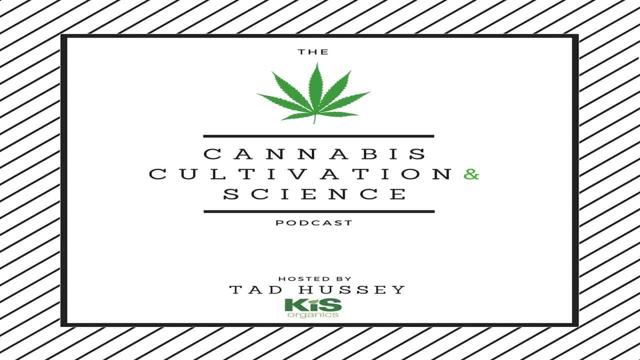 Well, currently I am working on a soil survey for heavy metals in Louisiana, But I'm not sure. But I always welcome samples from around the country. It's really interesting to see what people are getting in their soils or amendments or fertilizers. 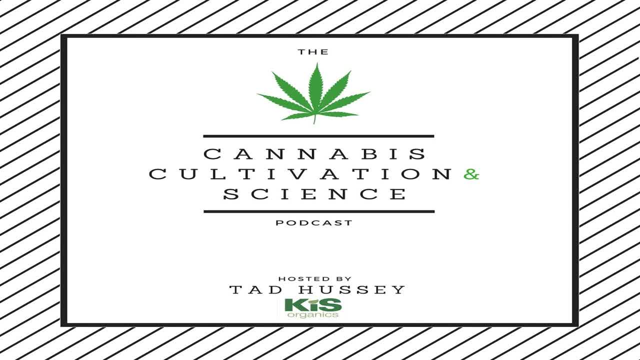 So lab is open to other people from across the country to send the samples to us. I continue studying heavy metals in a different form and shape And my current research also involves using magnetism- soil magnetism- to understand how that may correlate with heavy metals and also find a way to make methods even less time consuming, even more affordable. 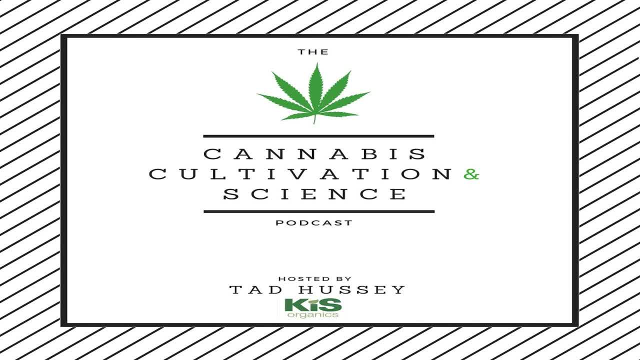 So we're still working on developing the best methodology possible And hopefully in the future we'll be able to offer the bioaccessibility test with XRF. So we are still working on that. We'll make it through portable technology. So yeah, basically, if people want to send their soils to the lab, feel free to send them to our website or just Google Delta Urban Soils Laboratory. 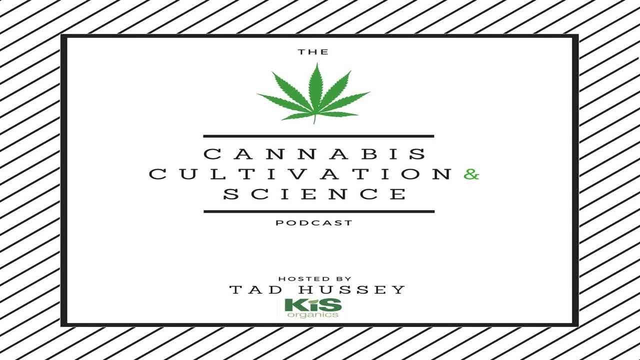 And they will find information on how to collect their samples and where to mail them to. And if they want to look at my research, I also have my website- It's Anna Pelceva- Annapelcevacom, And my Instagram Soil Underschool Expert. 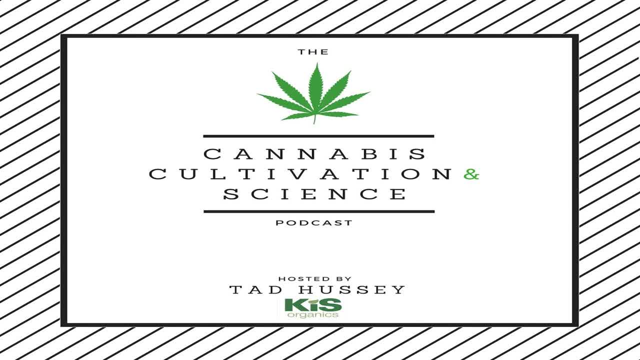 I love chatting with different people and I always respond on my Instagram, So I'm going to be pleased to hear what people experience in their gardens and homes around the country. Absolutely, I'm glad you brought those up, because I was going to list all of those things. 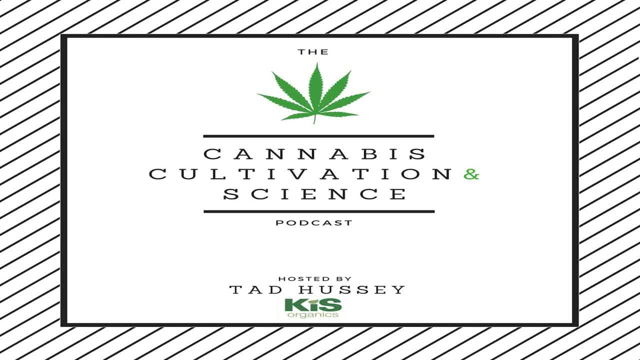 And I'll have them in the introduction as well and on the podcast page Because it might be a little tricky to do. It might be a little tricky to spell your last name for people unfamiliar, But I highly suggest people do check out your social media. 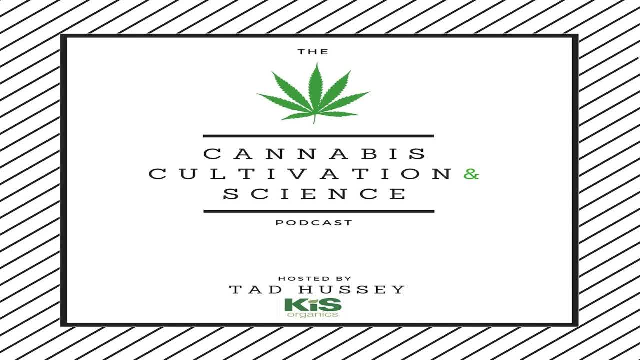 You're quite active on there And you just recently posted- I saw- a story where you were showing exactly how you do the testing on the heavy metal analysis, which I thought was fascinating. It's wonderful to actually see what's happening in a lab. 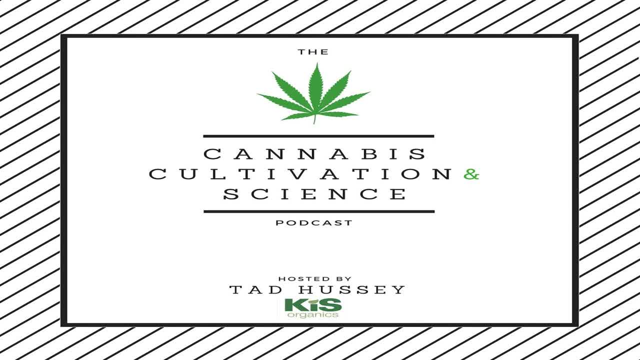 And you're a very interesting mix of fashion And soil science which you don't typically put together. So I think it's a lot of fun And people should definitely check you out. Thank you so much. I appreciate that you reached out to me and invited me to the podcast. 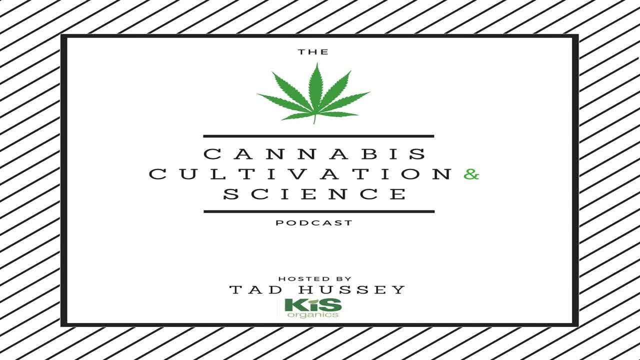 And I'm excited to collaborate more on different projects, test more of your samples and be engaged with the audience. Yeah, We definitely will be sending you a lot more samples as we try to discover, not just tests. We're in the process of testing all of our soil amendments and fertilizers right now to make sure that we know the heavy metal levels and know that they're safe.